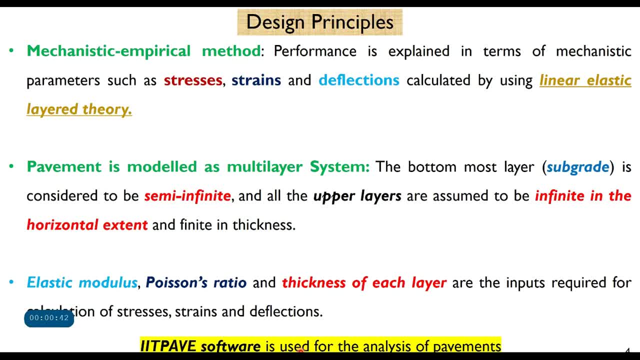 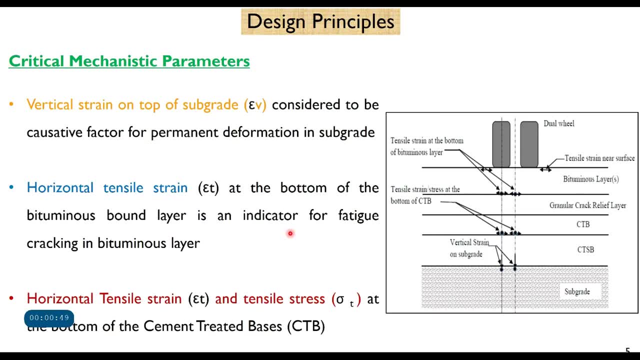 NIT software is used for the analysis of the pavement. Now the critical parameters which are considered in the design of a flexible pavement are: 3. Vertical strain at top of subgrade. that is considered to be a causative factor for permanent deformation in subgrade, or you can say rutting The horizontal tensile strain at the bottom. 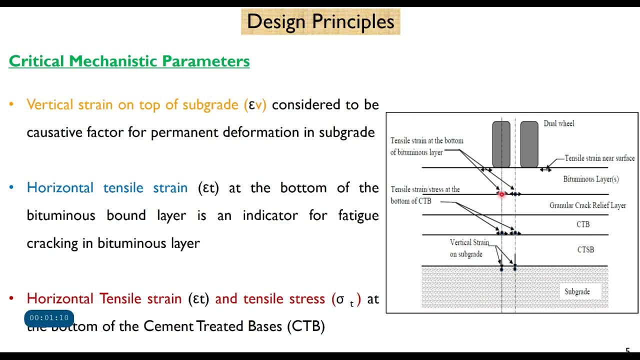 of the bituminous bound layer and that is the indication of permanent deformation in subgrade or you can say rutting The horizontal tensile strain at the bottom of the bituminous indication of fatigue, cracking in bituminous layer and horizontal tensile stress and strain. 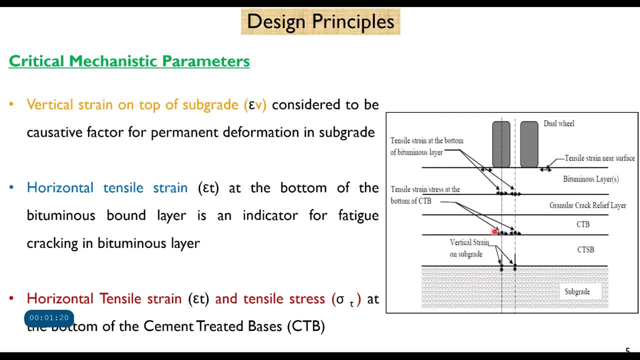 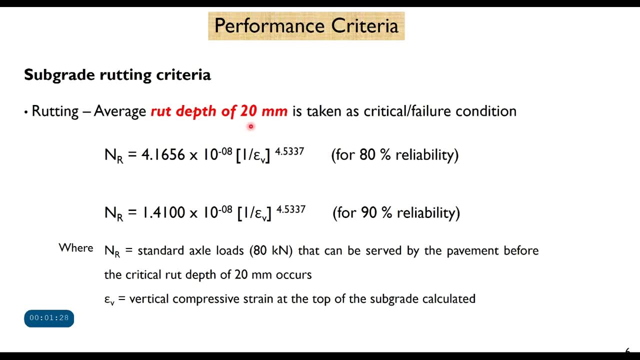 at the bottom of the cement treated base. The subgrade rating criteria given in IRC 37 is that if rating is 20 millimeter or more, that is considered to be the failure condition, means the pavement has failed and if you calculate the vertical strain- compressive strain at top of. 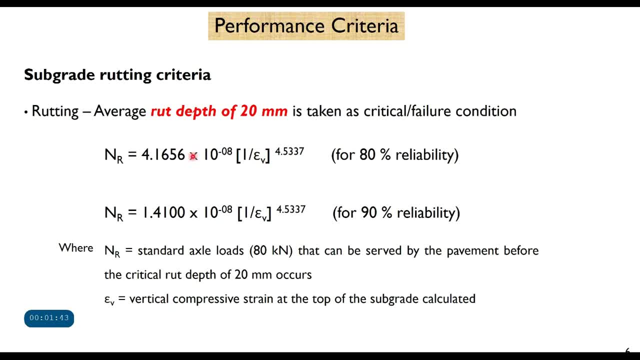 subgrade. using IIT-PAVE, you can find out how many repetitions, how many repetitions of standard axial load this pavement can take. Alternatively, you can you know the design traffic and, corresponding to this design traffic, what should be the permissible value of epsilon v, that is, vertical. 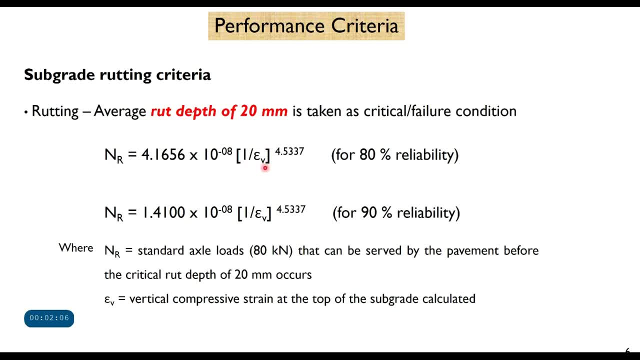 compressive strain and you design a pavement so that this strain is less than the allowable strain. This equation is used for 80% reliability and this equation is given for 90% reliability. Now, reliability here means the ninety percent chances are that the pavement will last its design. 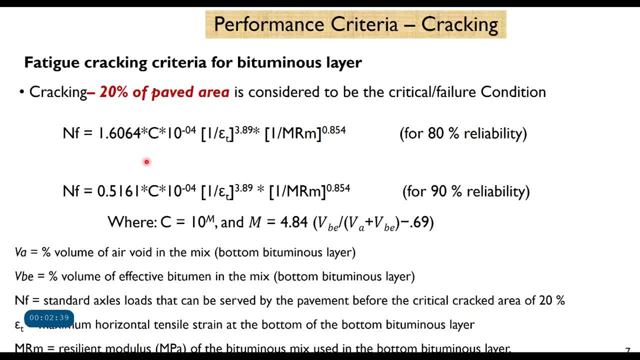 life. The fatigue criteria which is considered in the design is that if 20 percent of paved area is cracked, that is considered to be the failed condition. and here this is the tensile strain at bottom of bituminous layer and this is the resident modulus of the bituminous. 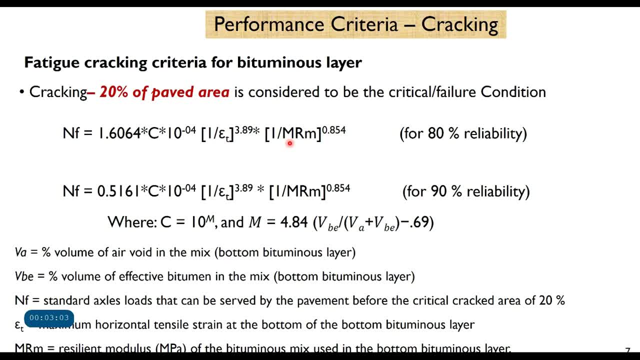 mix used in the bottom bituminous layer. if you are putting two layers of bituminous mixes, then bottom layer should be considered and the again. there are two equations here for 80 percent reliability and for 90 percent reliability. we should use for for nh and state highway and express. 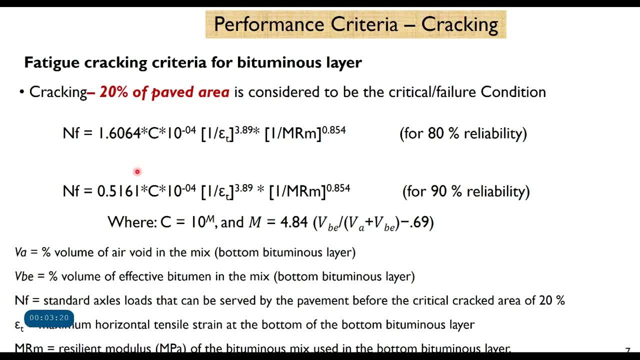 way we use 90 percent reliability equation here. c is a parameter which is given by this 10 to the power m, and m depends upon the mix condition and that's the departure uh in this code from earlier code that here we consider the mixed design parameter also while calculating the fatigue life. 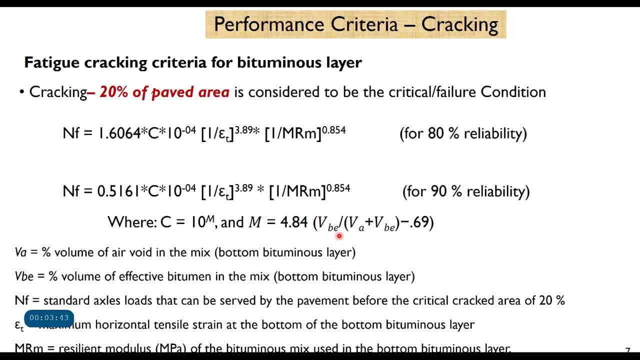 of a pit. This is the effective binder content and va is the air wires in the mix. so from this we calculate m, from m we calculate c. put the value of c here and the tensile strain at bottom of bituminous layer and mr value of the bituminous mix and you can calculate how many. 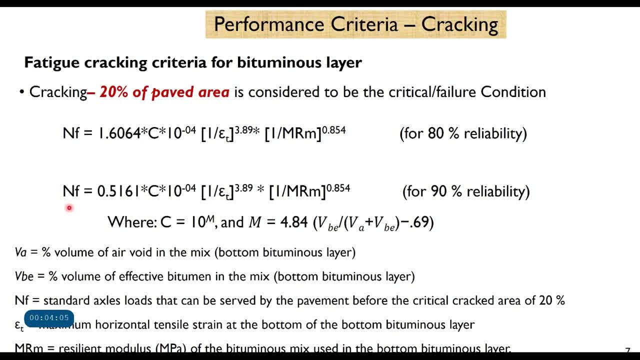 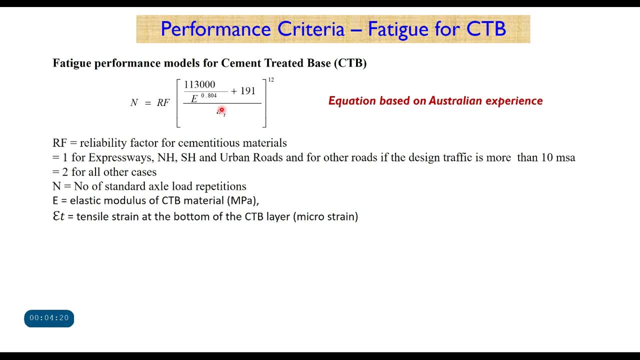 cycles it can take or how many repetitions of standard excel load this pavement can take before the critical crack area is 20 or more. for cement treated base, there are two considerations. one is based on tensile strain, another based on tensile stress. this equation is based on australian experience. 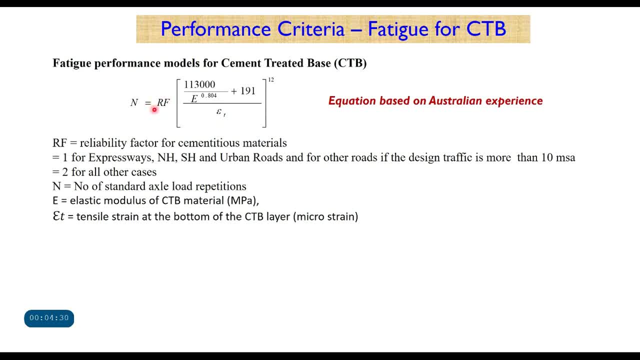 and here the rf is the reliability factor, which is one for expressway, national highway, state highway and urban roads, and for other road also if the end traffic is more than 10 msa. 2 for all other roads. n is the number of standard excel load repetition, e is elastic modulus of. 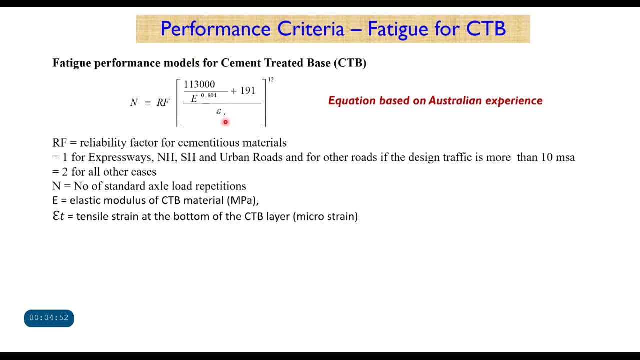 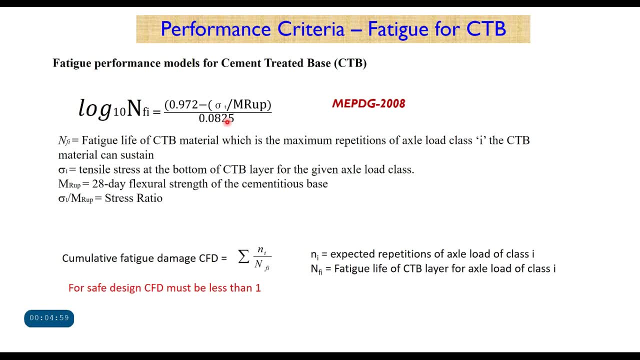 ctb material, and this epsilon t is tensile strain at bottom of the ctb layer. now another parameter here is based on the stress sigma t. here is tensile stress at the bottom of ctp layer for given excel load class. so here we determine what is the fatigue life of ctv material for a particular load class. 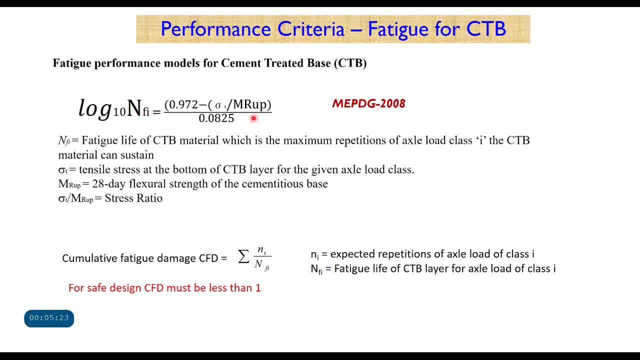 i and this mrup is 28 days. flexible strength of cementitious base and the sigma t upon m rup is called the stress ratio. from that you determine the cumulative fatigue damage. cfd summation of ni upon nfi, and this value should be less than one. 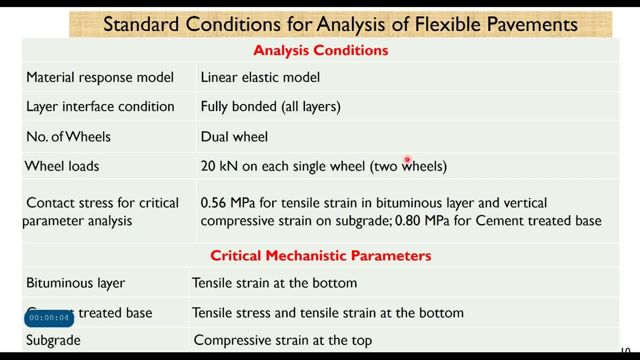 so extended conditions which are taken for the design of flexible pavement are that material response model is considered to be linear, elastic. the interface condition is fully bonded. number of wheels: dual wheel and wheel load is 20 kilometer on each single wheel, that is, two wheels. contact stress: 0.56 mpa for tensile strain and bituminous layer and vertical compressive. 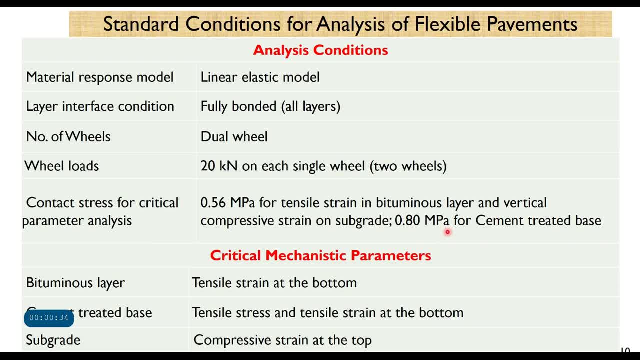 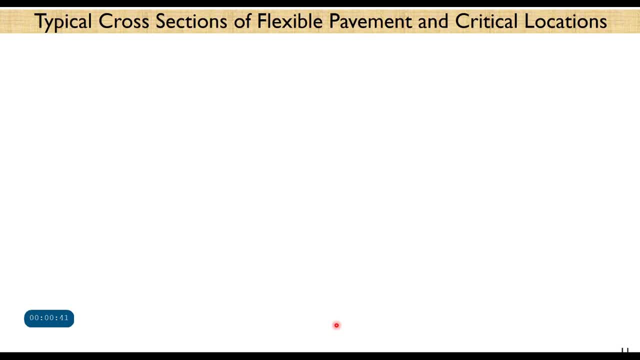 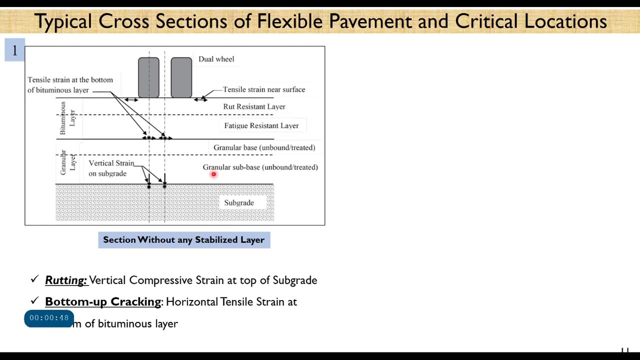 strain on subgrade and 0.8 mpa for cement treated base. and these three condensate are critical, as i explained to you earlier. also now, let us say you take a very conventional pavement where you have subgrade, granular subbase and base and then you have bituminous layer. now, in this case, there 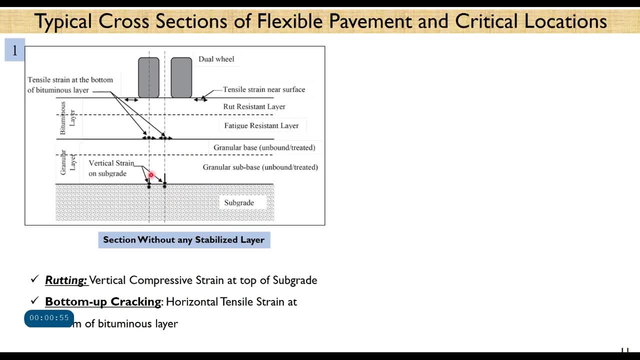 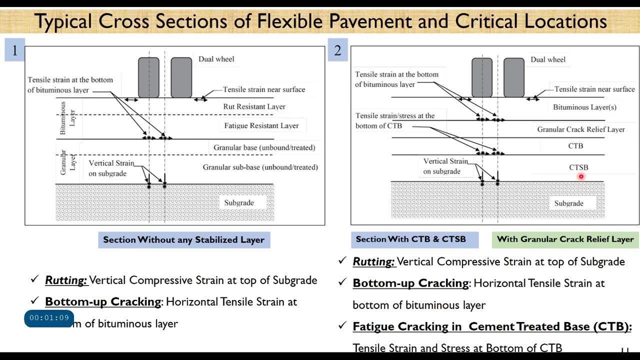 there are only two critical conditions. One is the vertical strain on subgrade top of subgrade and tensile strain at the bottom of witness layer. Only these two conditions are critical. But when you have the CTSB cement treated subbase, 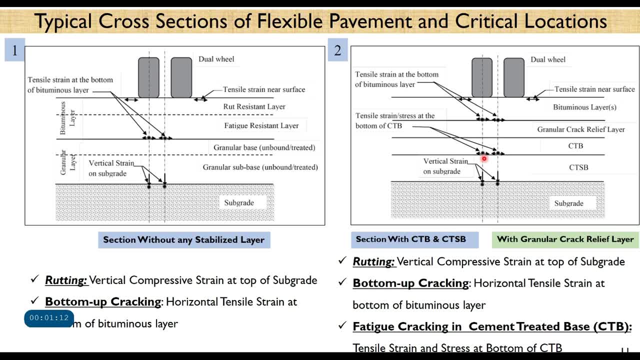 and cement treated base, then these three conditions are critical: The vertical strain on subgrade, the tensile stress and strain at the bottom of CTB layer and tensile strain at bottom of witness layer When you have a cross section where CTB and CTSB are used. 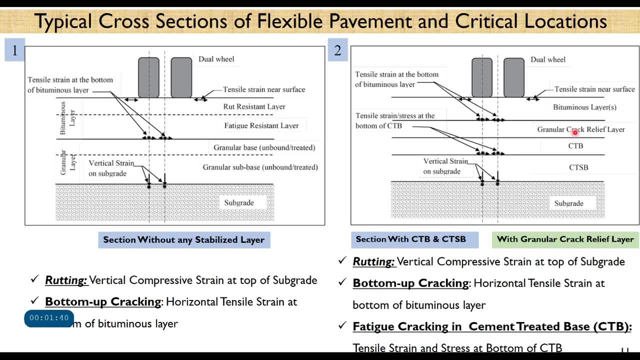 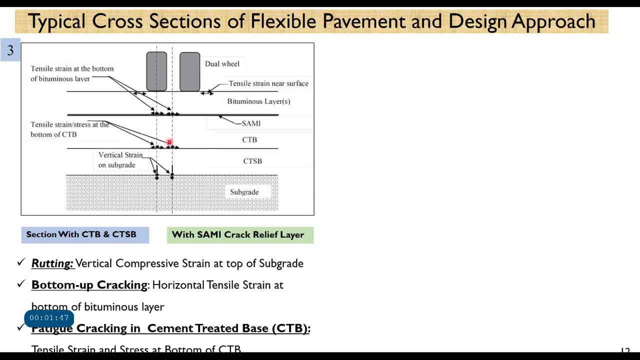 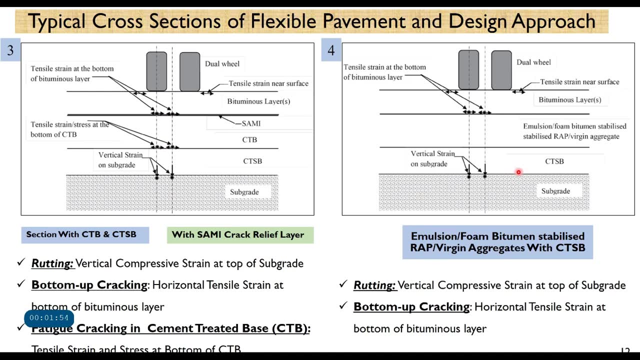 but rather than providing the granular crack relief layer, you are providing the semi layer. then also the condition remains same. All three conditions are critical conditions. When you have emulsion or form bitumen stabilized base, then in that case the critical conditions are only two. 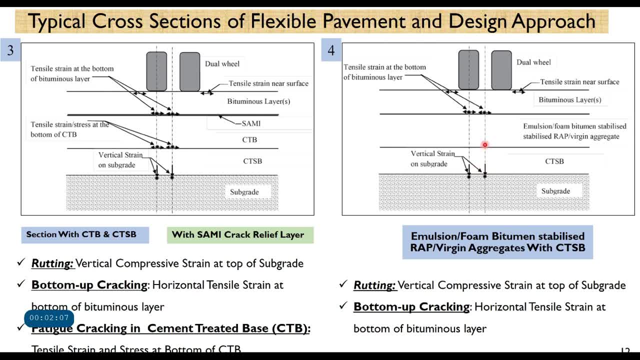 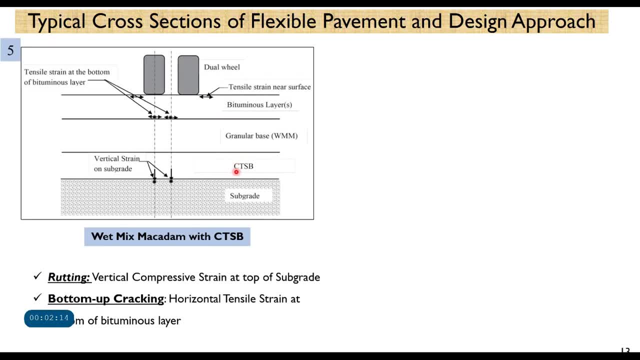 The vertical strain on subgrade and tensile strain at the bottom of witness layer. In case of CTSB, that is, cement treated subbase, then only two conditions are critical: The vertical strain on subgrade tensile strain at bottom of witness layer. 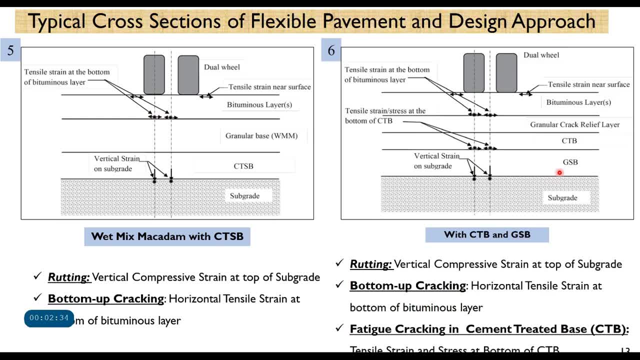 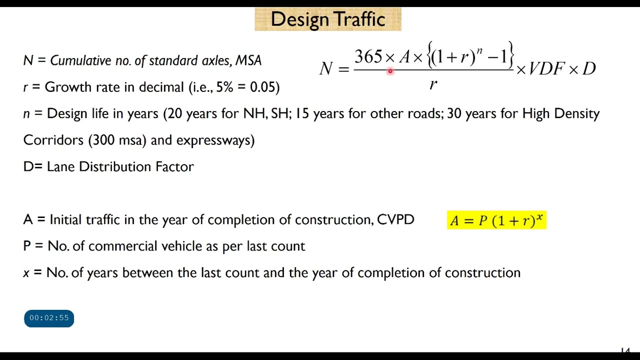 But when you are providing GSB- granular subbase in the subbase course and above that you provide CTB and then a granular crack relief layer or semi, then all three conditions become a critical condition conditions. The design traffic is calculated using this equation, where A is initial traffic. 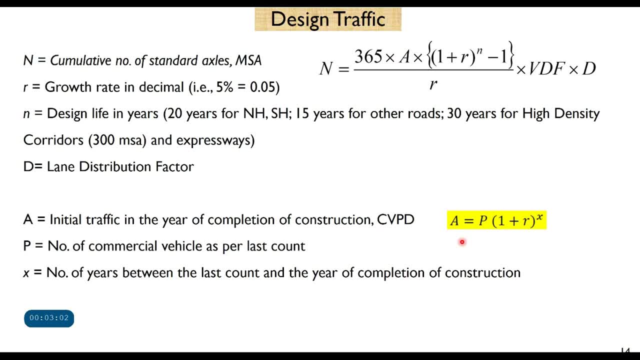 in the year of completion of construction, and that, basically, is calculated using this equation, where P is the number of commercial vehicles as per last count, R is the growth rate of the traffic and X is the number of years between the last count and the year of completion. Now here, VDF. 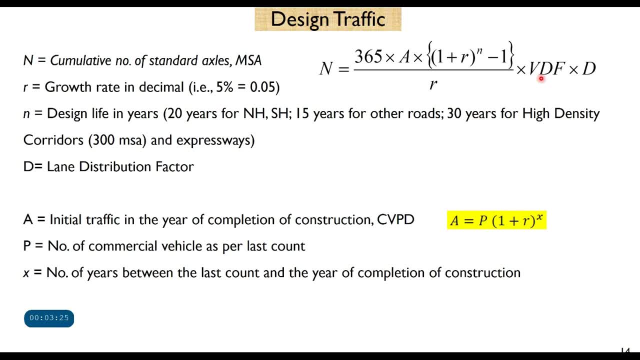 is the vehicle damage factor and D is the lane distribution factor. For understanding this vehicle damage factor, you can see my another video on how to calculate VDF, and link for this is given in the description box. Lane distribution factor depends upon the type of carriageway. 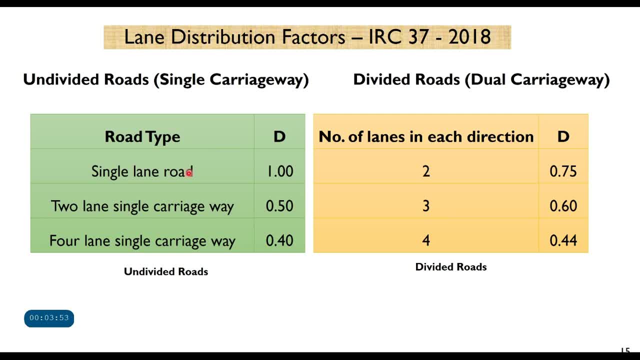 if it is single carriageway: single lane road it is 1,. 2 lane single carriageway it is 0.5 and 4 lane single carriageway it is 0.4. and similarly for dual carriageway for divided highways, these lane 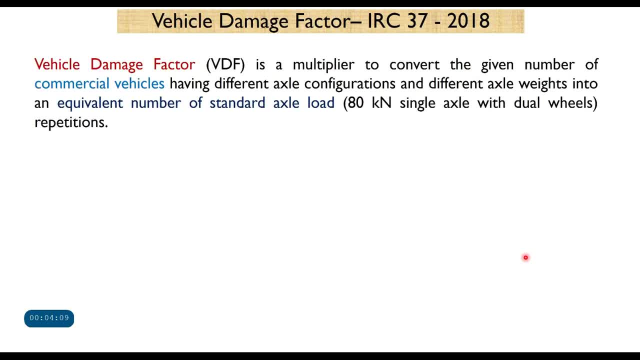 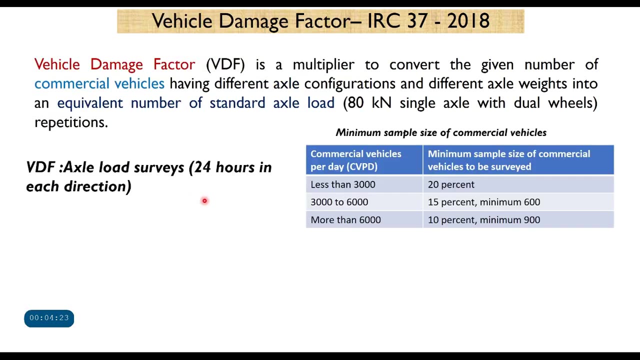 distribution factor can be taken from this table. The vehicle damage factor is a multiplier to convert the given number of commercial vehicles having different excel configuration and different excel weights. I will not go into much details of this because this point I have already explained in one of earlier videos and you can refer that video for further details. 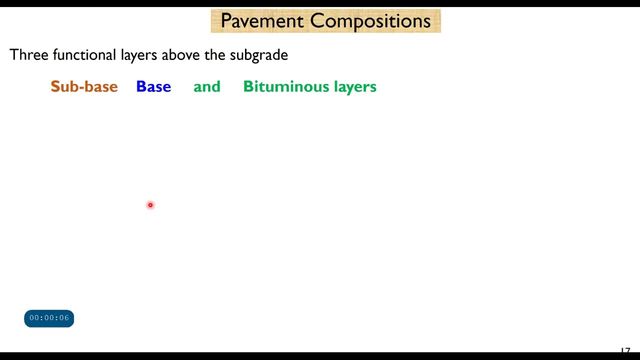 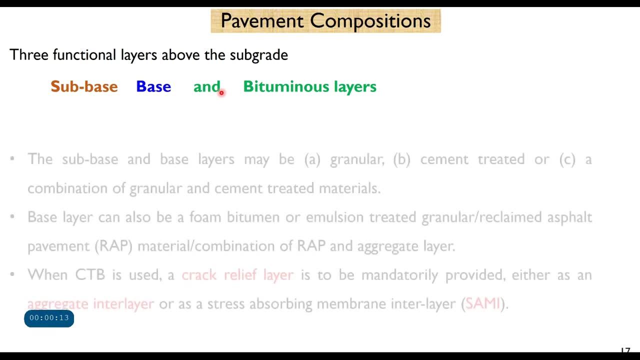 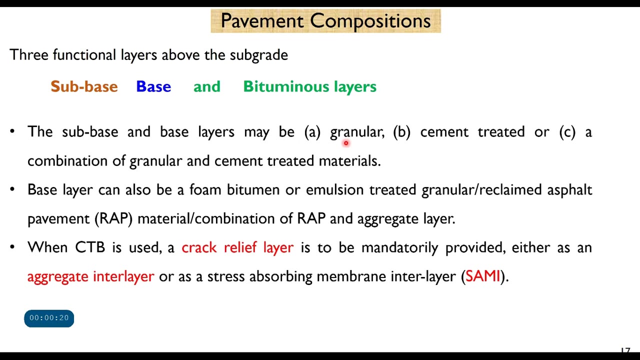 A flexible pavement will have three functional layers on most sub grids: sub basin, base and bituminous layers. Now, the sub base and base layers may be granular or cement treated or a combination of these two. Similarly, base layer can also be a form bitumen. 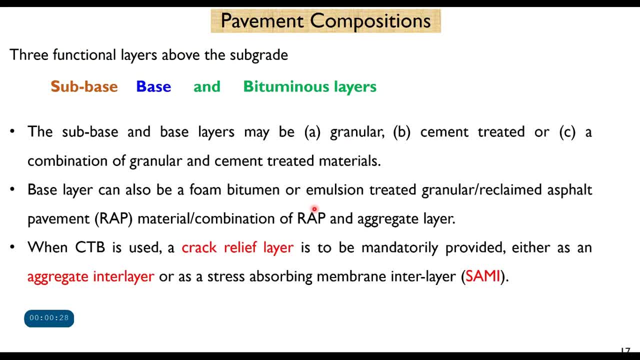 or emulsion treated material, or it may be wrap material or combination of their or their combinations. When cement treated base is used, a crack relief layer is mandatory to provide. This can be either in the form of aggregate interlayer or it can be in the form of a semi-layer. 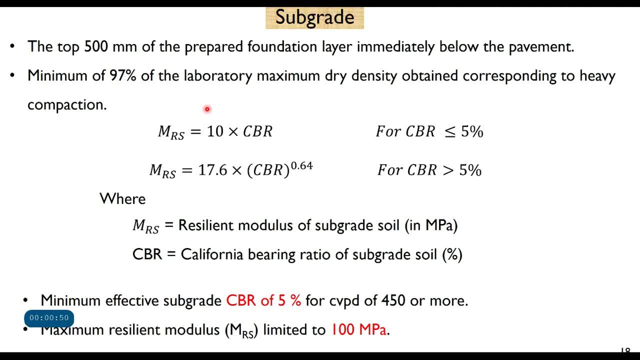 The top 500 mm of prepared foundation layer immediately below the pavement is called the subgrade, and the input parameter required for subgrade in IID-PAVE is resident modulus. and resident modulus can be estimated from the CBR value using these empirical equations given in the IRC code. 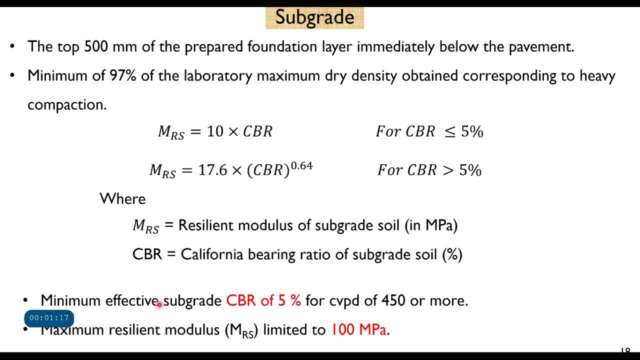 When the subgrade is prepared in a sub-grade, it is a subgrade that is calculated in the rooms in the sub-grade and in the sub-grade it is calculated in a sub-grade, The sub-grade prepared using a material which is stronger than top 500 millimeter of. 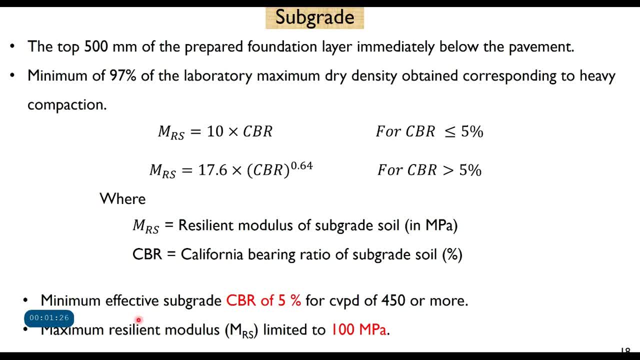 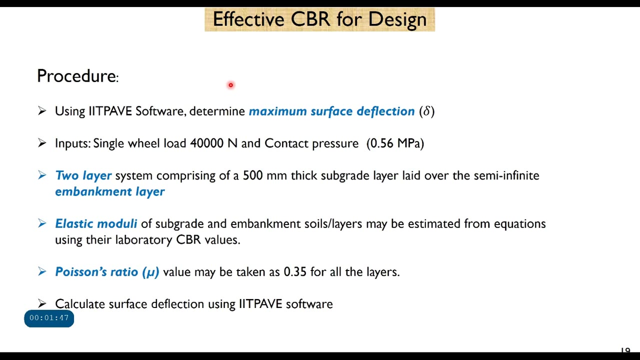 embankment soil, then it is important to estimate effective CBR, which will reflect the contribution of both of these materials And the maximum region modulus of subgrade is limited to 100 mPa. Now how do we determine effective CBR in case subgrade is provided on embankment and the soil used for 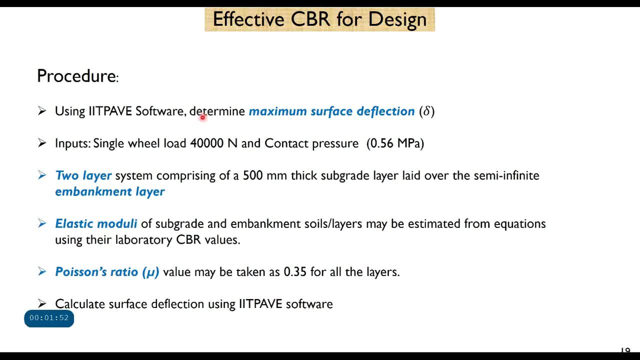 embankment and subgrade are different. So first we calculate the maximum surface deflection from IIT-PEF software, and for that input parameter will be single wheel load of 40,000 Newton and contact pressure of 0.56 mPa. It will be a 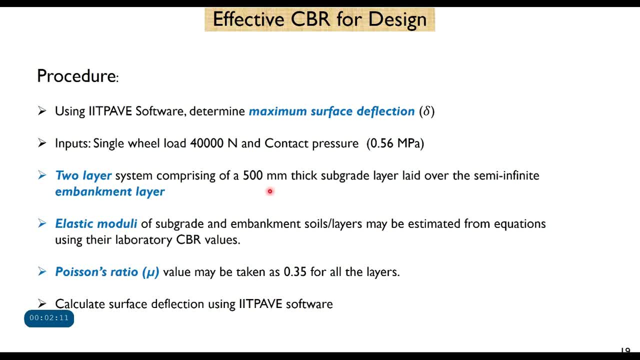 two-layer system where 500 millimeter thick subgrade layer layers over semi-infinite embankment layer. But in case of embankment layer also we take only top 500 millimeter thickness, Means we considers CBR of the soil which is used in top 500 millimeter of embankment, Calculate elastic moduli of: 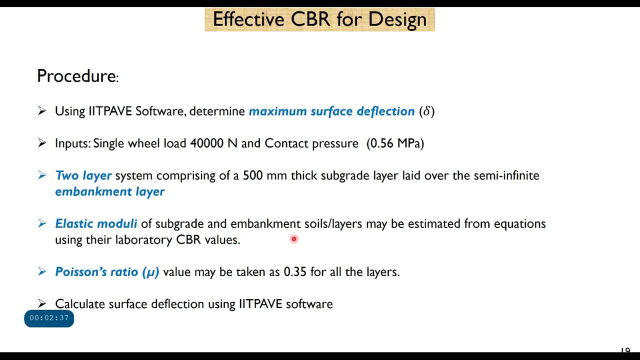 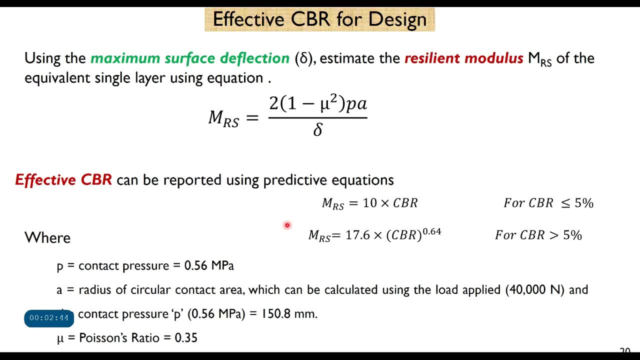 subgrade and embankment soil. from the equation Potential ratio can be taken: 0.35 for all layers, and we calculate the surface deflection. Now the surface deflection is used to calculate the resilient modulus. This is the resilient modulus of equivalent single layer And if you know, MRS, value. 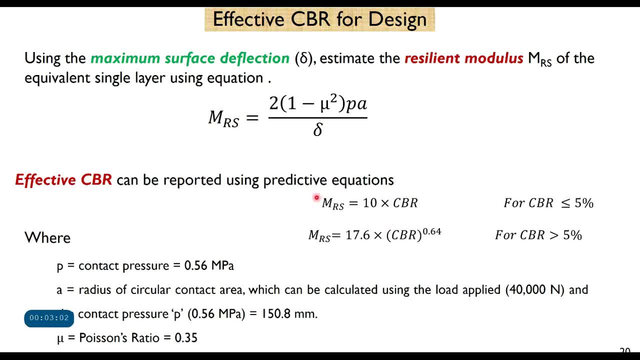 you can find out what will be the CBR effective CBR using one of these two equations, depending upon the value of CBR. In this equation, small p is a contact pressure which is taken 0.56 mPa. a is the radius of circular. 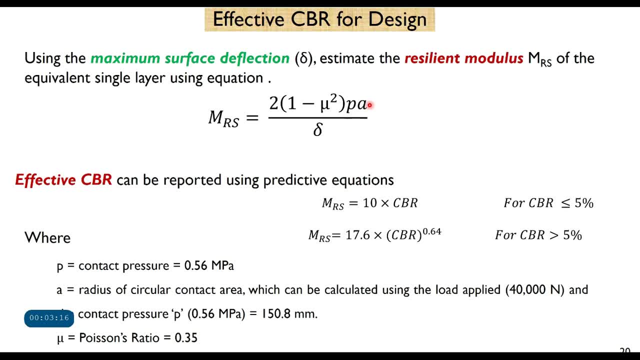 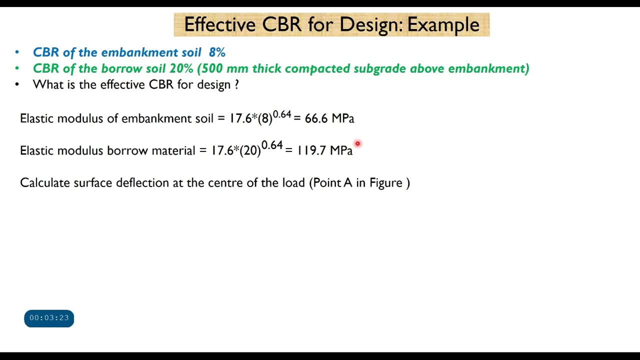 contact area, which is taken as 150.8 millimeter, and mu is the Poisson ratio. Now let us take one example to demonstrate how effective CBR is calculated. An example is that CBR of the embankment material is 8% and CBR of the 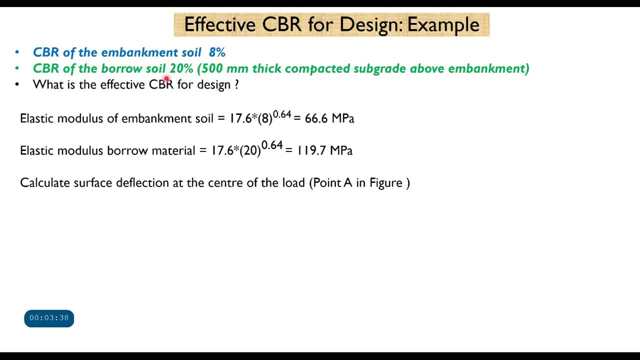 borer soil which is used to prepare subgrade is 20%. So what is the effective CBR for the design? CBR of the embankment material is 8% and CBR of the borer soil which is used to prepare subgrade is 20%. So what is the effective CBR for the design? 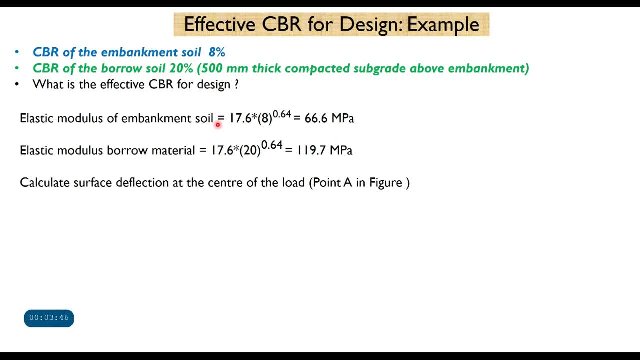 For the design of embankment soil. we determine what is the value of elastic modulus using this equation, because it is more than 5% and therefore we'll use 17.6 into CBR, the power 0.64, ie 66.6 mPa. 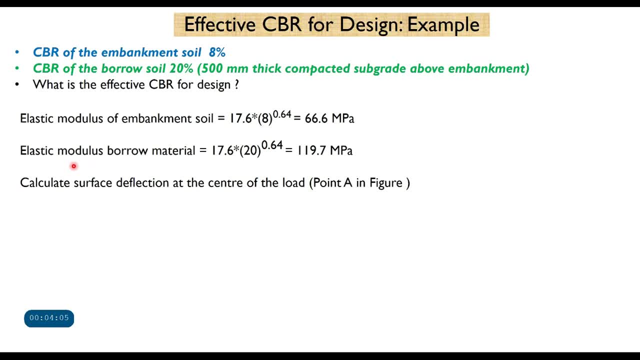 The elastic modulus of borer material is 119.7 mPa. Now this is the structure. you have two layers, the embankment has semi-infinite thickness and above that you provide 500 millimeter thickness of subgrade soil, and these are E values. So with these values, we 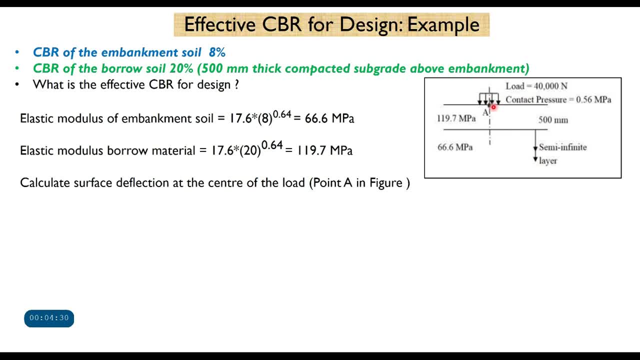 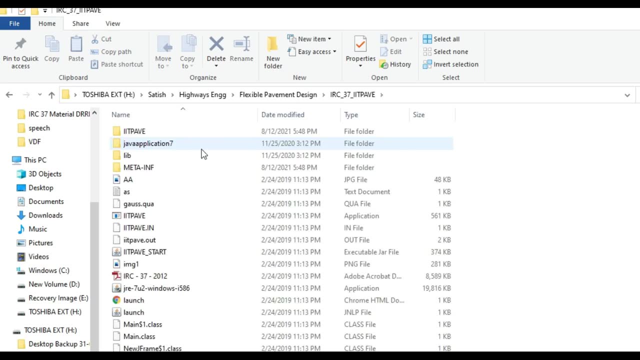 calculate what is surface deflection using IIT-PAVE. Now let us go to the IIT-PAVE to illustrate this procedure. how do we find the surface deflection? This is IIT-PAVE software on my system. You just click it, First thing you have. 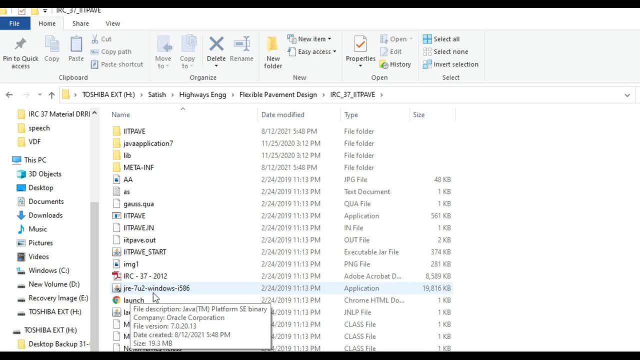 to do, you have to install Java. So this file, JRE7U2, window 586, is to be clicked and then it will install Java on your system. Once it is done, then you can start this IIT-PAVE start. So when you double click this software, 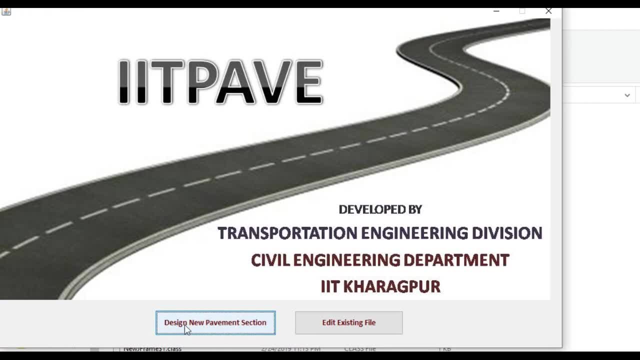 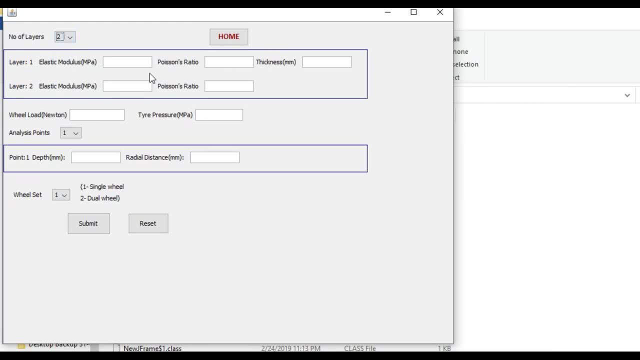 here you say design of new pavement, and then so here you will say number of layers: 2 and fill the values of elastic modulus. The first layer is your subgrade. therefore E value is 119.7.. The Poisson ratio is 0.35.. Thickness is 500. 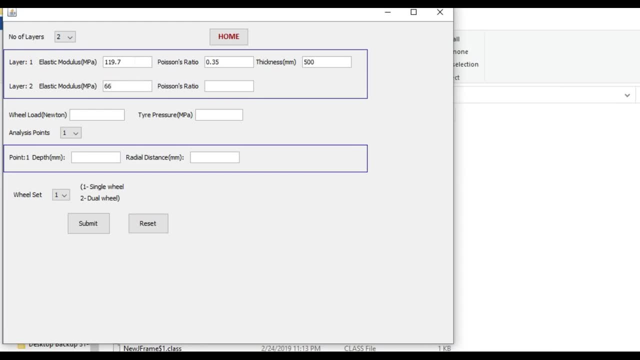 millimeter. The second layer E value is 66.6. that is your top embankment Poisson ratio, same: 0.35.. Wheel load is 40,000 and tire pressure is 0.56.. We need only one analysis point, and that is the. 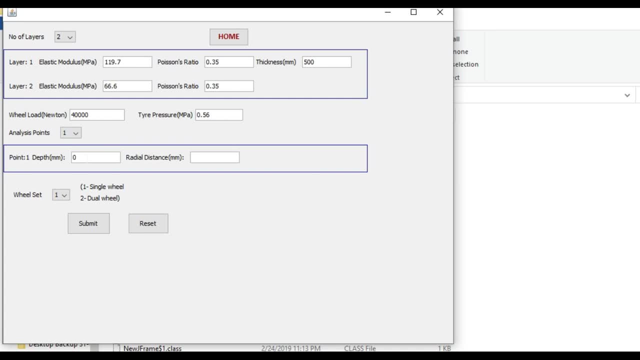 surface deflection below the load and therefore depth will be 0 and radial distance will also be 0. So if you submit these data, it says submitted successfully And then you run the program. So when you run the program you can view the file. 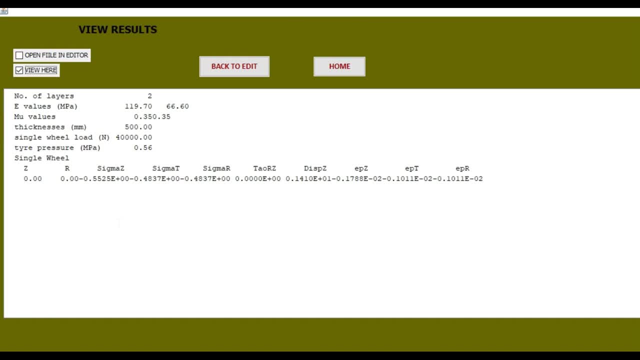 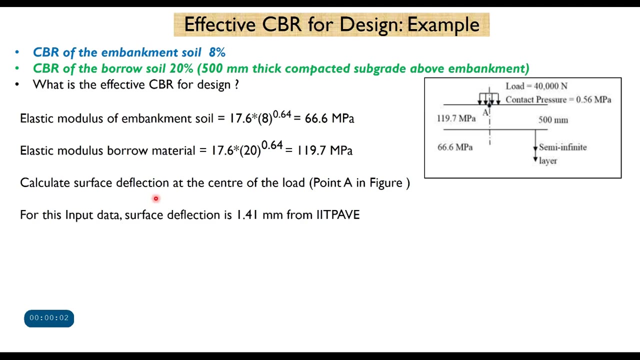 here. This is the complete file. So what is required here? Displacement Z, that is, surface deflection 0.141, into 10 power 1, that means 1.41 millimeter. Now, the surface deflection as calculated from IIT-PAVE is 1.41 millimeter And 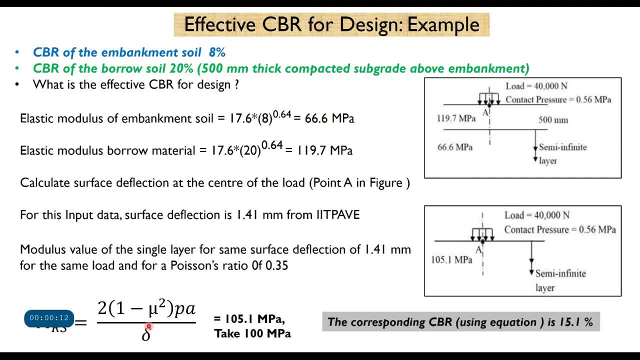 Here is the surface deflection ratio of E. We got one surface which is 0.35 millimeter T, which is approximately our surface deflection area, And what we have been able to achieve by this is that our surface deflection taken from four layers. 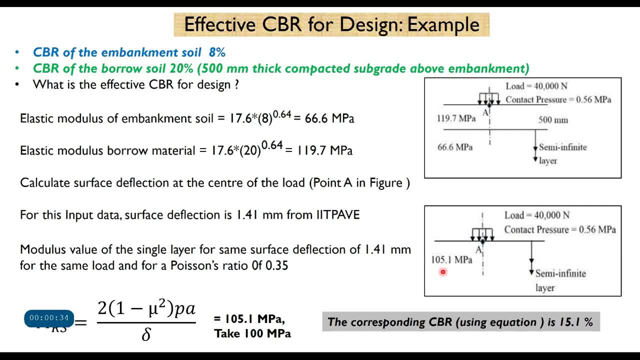 has been taken up by two layers And the surface deflection is about 0.48 millimeter. So this is the surface deflection, most of which will retainremos 6 meters. So this is pictures shown as a non- terra Bashar of our system. Here the surface deflection is License log. 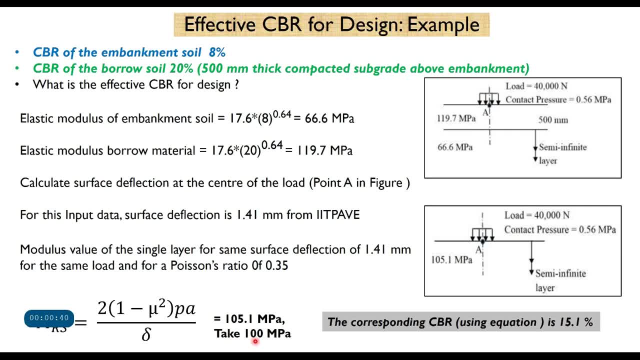 0. Kennel, So it is meant to be 0.15 minute, one of them. So as we calculate, mrs, that is 105.1 mg. maximum value of E can be only 100 MPa. So you take 100 MPa in this equation and you find out. 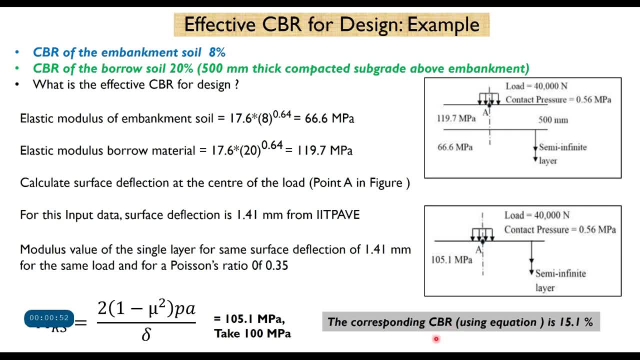 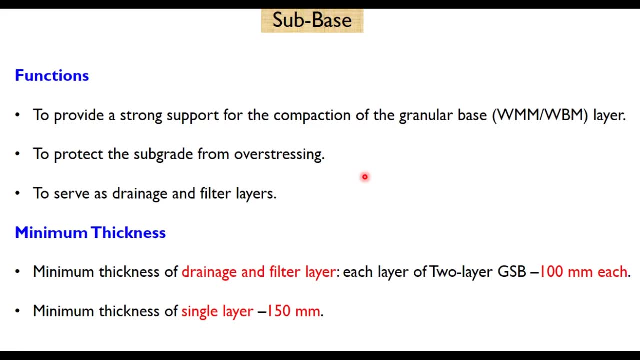 what is the value of the CBR? So you take 100 MPa and put in this equation and calculate what is the value of CBR. CBR is 15.1 percent and that is the design CBR. After subgrade we prepare the. 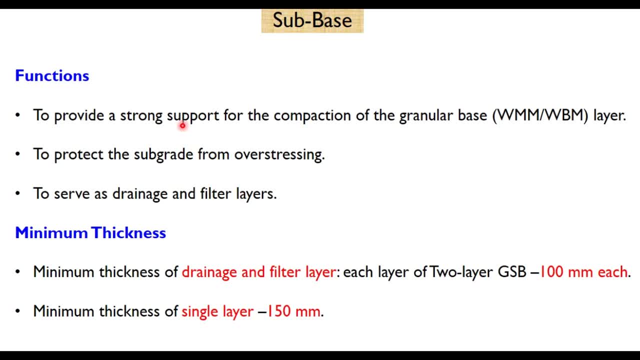 subbase and functions of subbase, as you all know, is to provide strong support for the compaction of granular base, to protect subgrade from over stressing, and it also serves as drainage and filter layers. When the subbase is provided in two layers, then the first layer will act as the 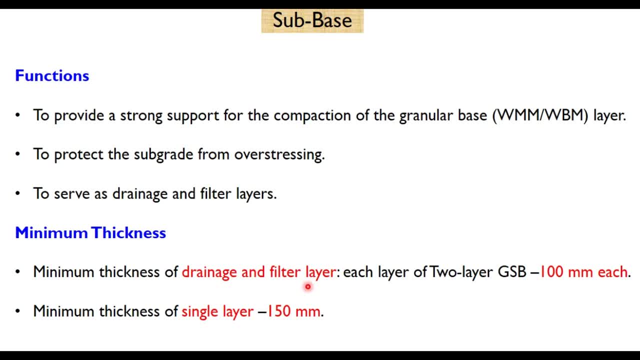 drainage layer and the lower layer will act as the filter layer. In that case, each layer should be at least 100 millimetre thickness. If it is to be provided in a single layer, then minimum thickness of subbase should be 150 millimetre. 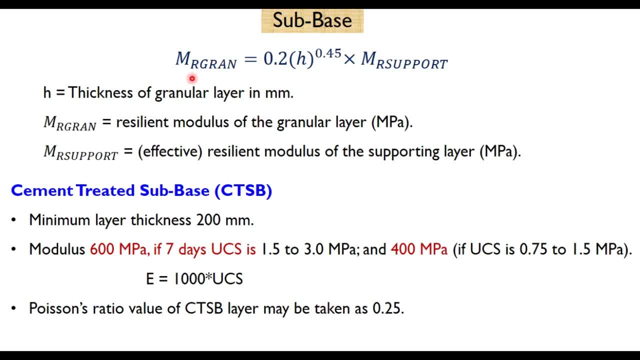 The MR value of subbase is estimated using this equation, where H is the thickness of granular layer in millimetre and MR support is the resident modulus of subgrade soil. That is the base support support provided by the subgrade. When we use cement treated subbase, then this minimum layer of CTSB should be 200 millimetre. 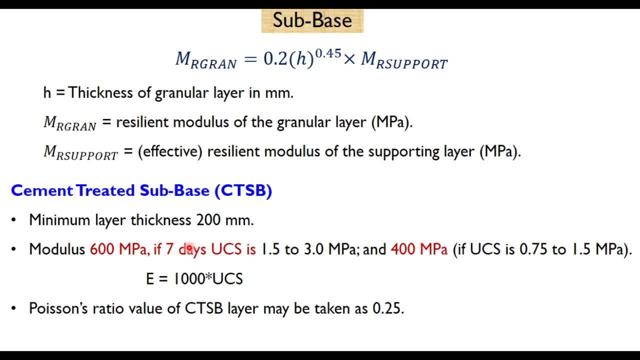 and elastic modulus can be estimated from the UCS test of the material and seven days UCS should be 1.5 to 3.5 millimetre. So this is the minimum layer of CTSB and the elastic modulus can be estimated from the material and 7 days UCS should be 1.5 to 3.5 millimetre. 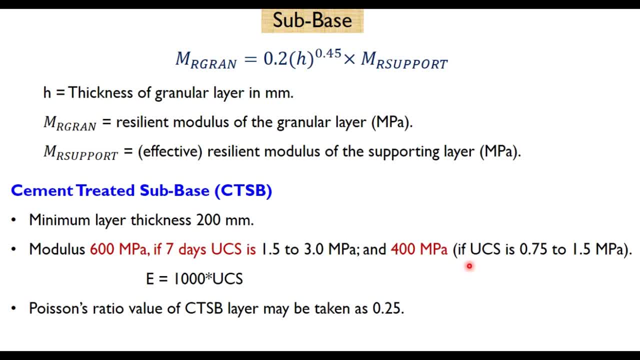 And if it is not for a weaker material, it can also be 0.75 to 1.5 ma. E value is estimated using this equation, 1000 times UCS, and this value, this equation gives you very high value- of E. CTSB is likely to crack under the construction equipment itself and therefore the 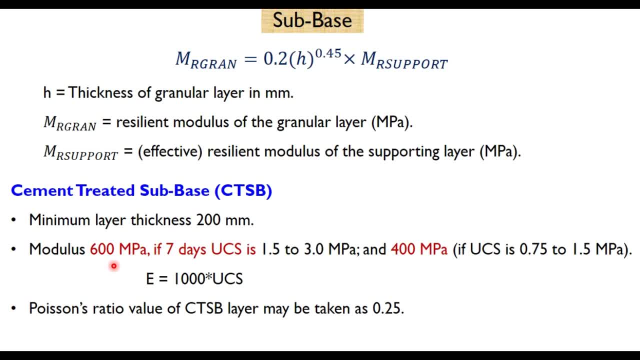 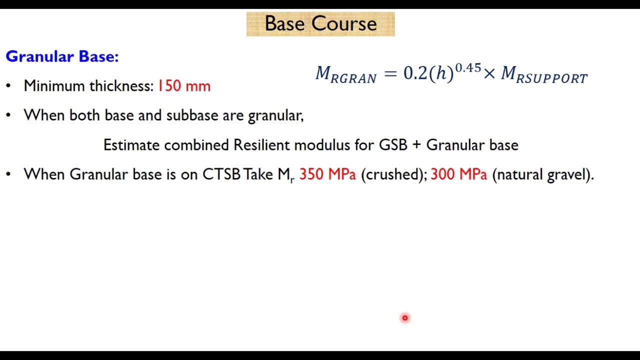 code suggests that the modulus value of CTSB should be 400 to 600 MPa and Poisson ratio for CTSB can be taken 0.25.. After the subbase we lay the base course and it can be granular base course. 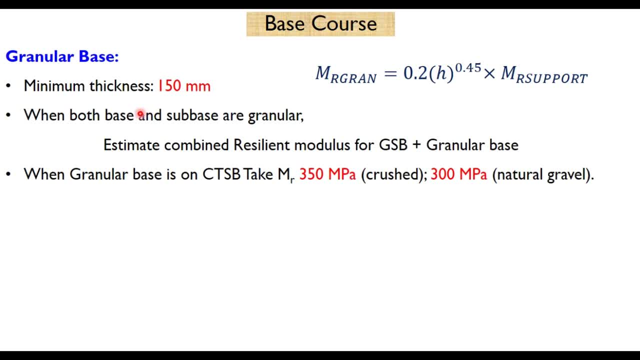 or it can also be cemented base course. When we provide a granular base course, the minimum thickness is 150 millimetre. when both base and sub base are granular, then we estimate combined residual modulus for GSB plus granular base and in this equation this thickness becomes the total thickness of sub base and base. 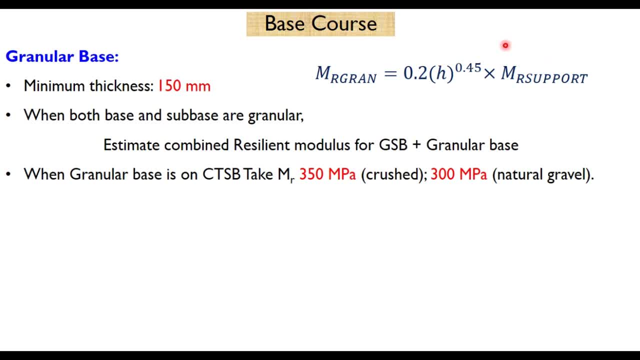 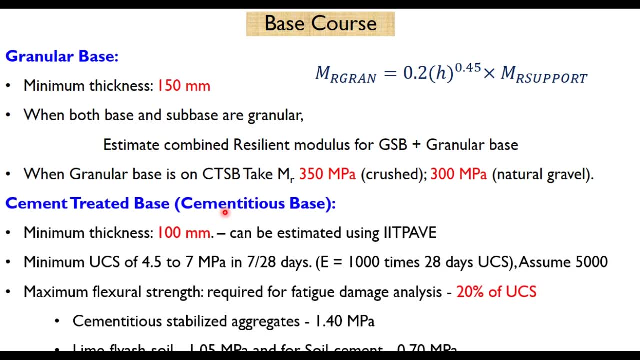 course layer and MR support will remain the modulus value of subgrade soil. When we use CTSB then we can take a graph of MR value of 350 MPa if it is of crushed aggregate and 300 MPa if it is natural gravel. 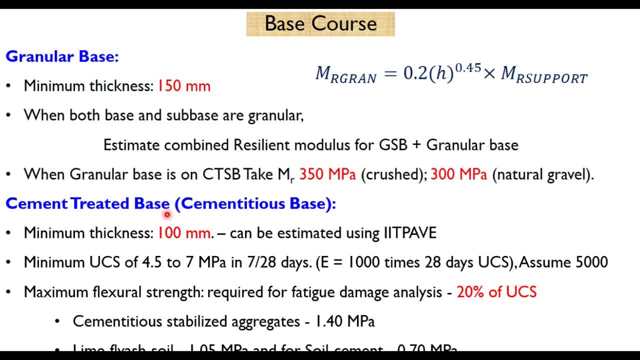 In case of cement treated base, the minimum thickness requirement is 100 millimetre and that can be estimated using IIT-PAV. The minimum UCS of the material which is to be used as cement cement treated base should be 4.5 to 7 MPa, and E value is again taken as 1000 times UCS. 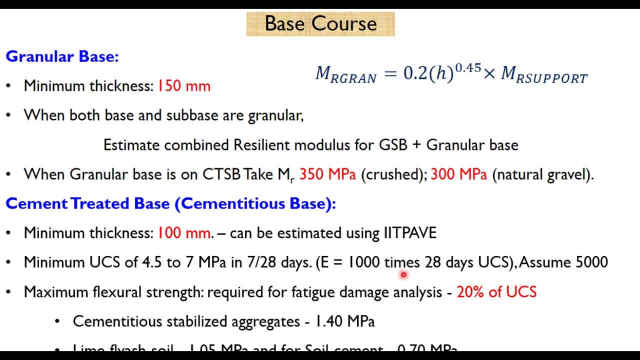 but what? the code suggests that the maximum value of E can be up to 5000 MPa. The maximum flexural strength required for fatigue analysis should be taken as 20% of UCS, subject to the following conditions: that for cementitious stabilized aggregate it should 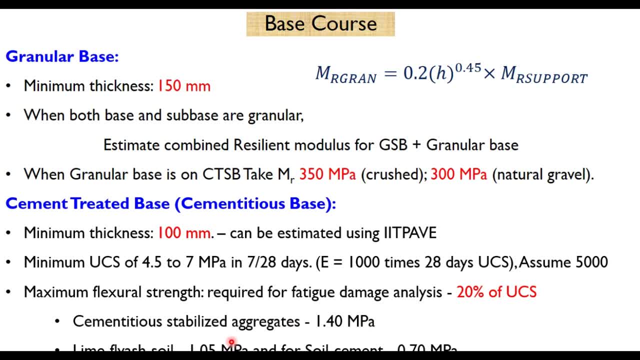 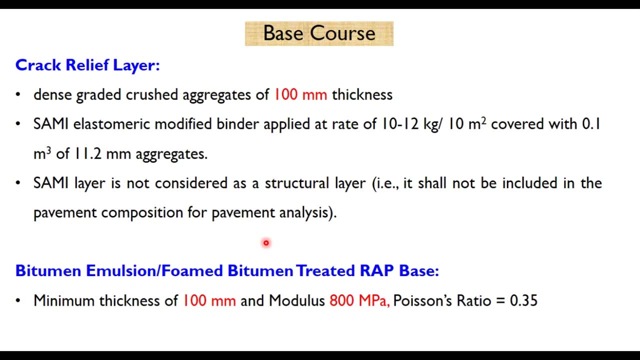 not be more than 1.4 MPa, and for lime fly ash soil 1.05 MPa, and for soil cement 0.7 MPa. In case of pavement with CTB, a crack relief layer between bituminous layer and the cementitious. 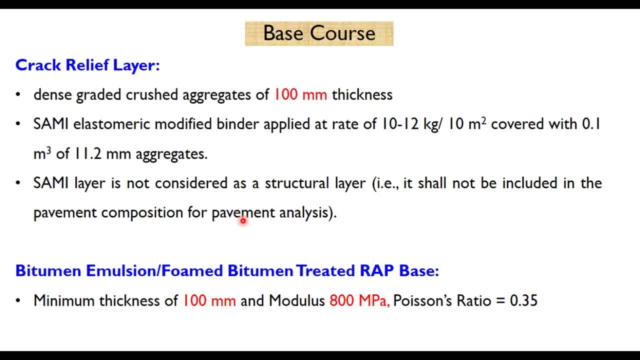 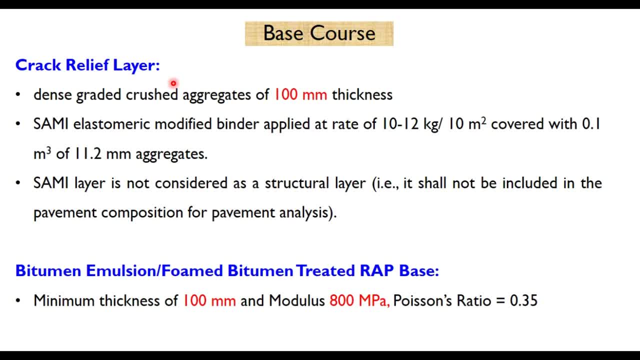 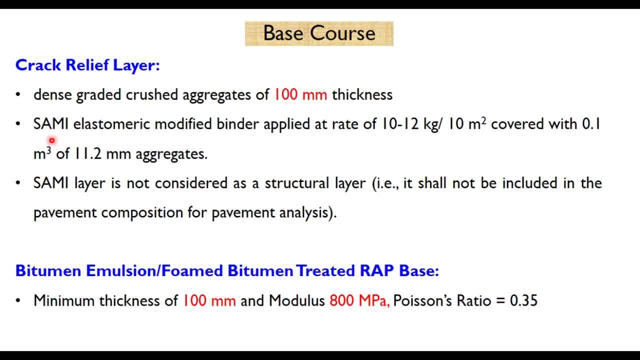 And therefore it is extremely important to provide crack relief layer between bituminous layer and cement touch base of 100mm thickness, or it can be a stress-absorbing membrane internal layer which is an elastomeric modified binder, applied at the rate of 10 to 12 kg per 10 m square covered with the carry-onяют 800° cerclated. 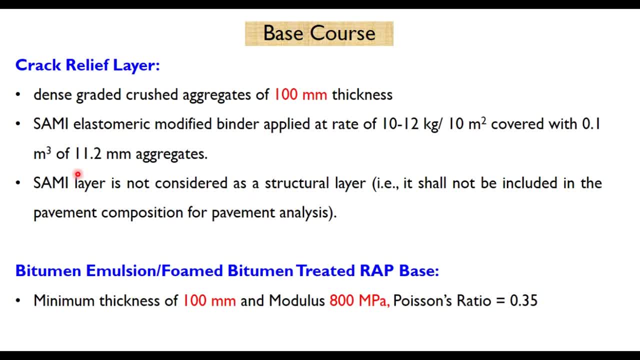 covered with 0.1 m3 of 11.2 mm aggregates. But when this is provided, when semi is provided, then it is not considered as a structural layer. That means it is not included in the pavement composition. The wrap material, with or without virgin aggregates treated with foam bitumen or bitumen emulsion. 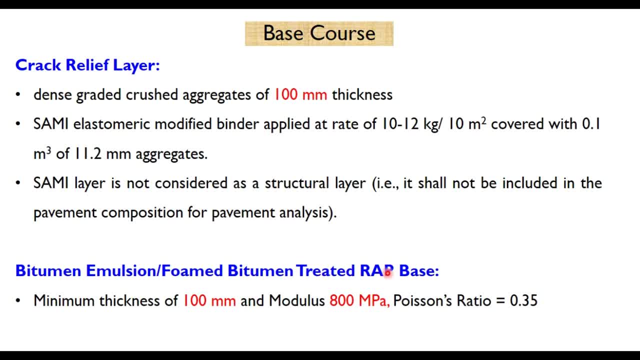 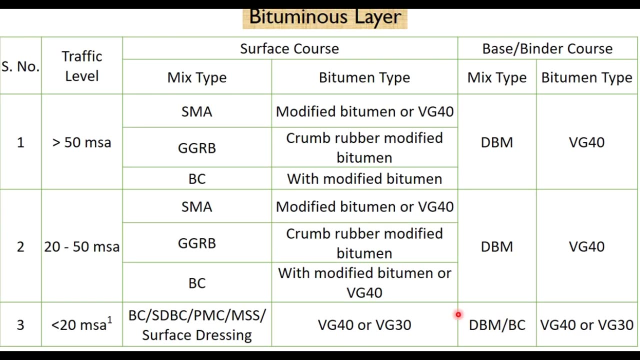 can also be used as base material, And in that case minimum thickness will be 100 mm and modulus value will be 800 MPa. The Poisson ratio for this can be 0.35.. Now bituminous layer is provided as per this table, depending upon traffic condition. 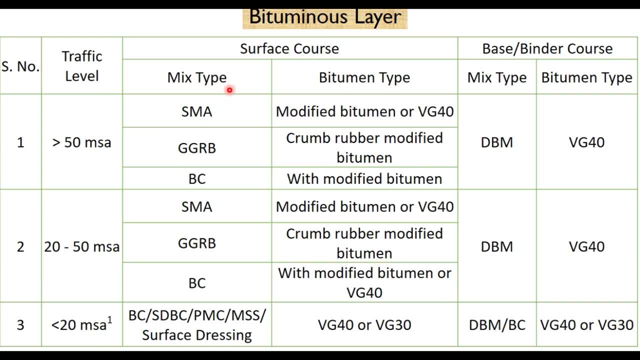 For 50 MSA or more. the mix type which is used in surface course can be stone matrix asphalt. It can be gap-glued, It can be graded mix with rubberized bitumen or bituminous concrete And corresponding binder course will be of DBM. 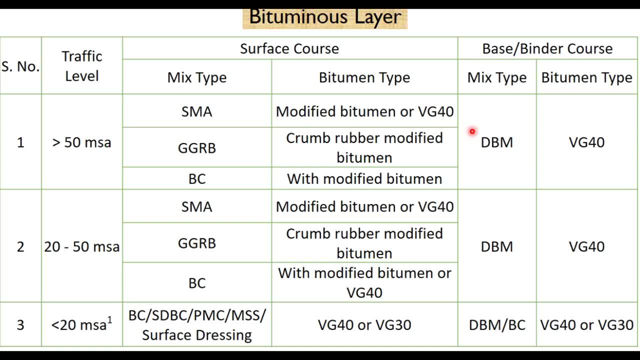 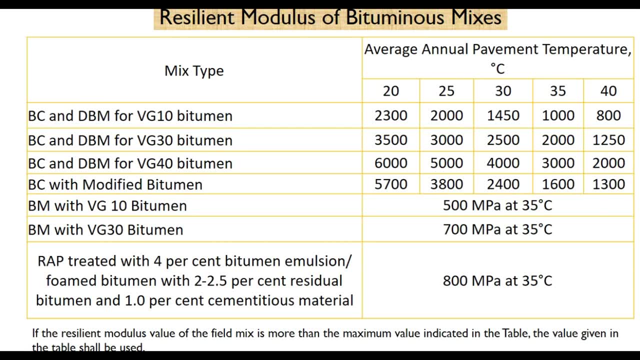 So this table can be used as a guide to select the type of binder course and surface course. The resilient modulus of bituminous mixes will depend upon the temperature and type of binder and type of layer, And this table is given in IRC code. 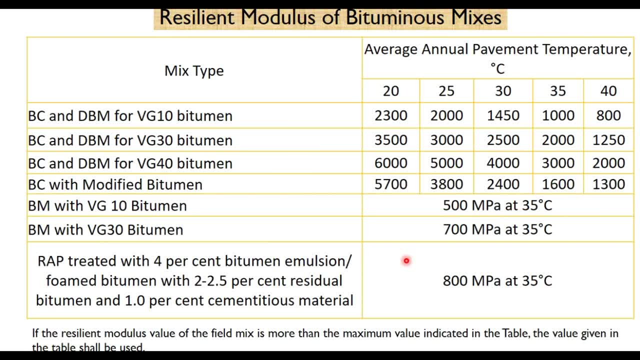 The design is required to be of the material, of the material, And the material is required to be of the material, of the material. Also, it is required to guide the designers to choose appropriate value of resilient modulus. It should be determined. as far as possible it should be determined in the laboratory. 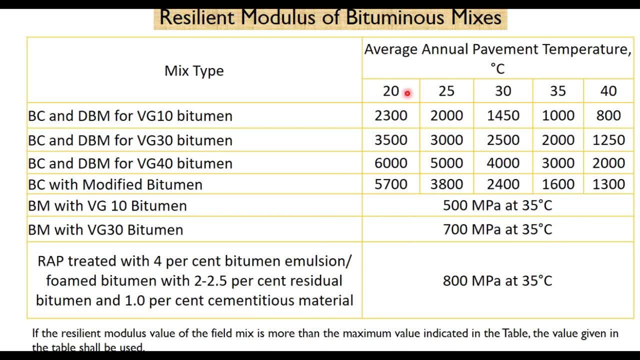 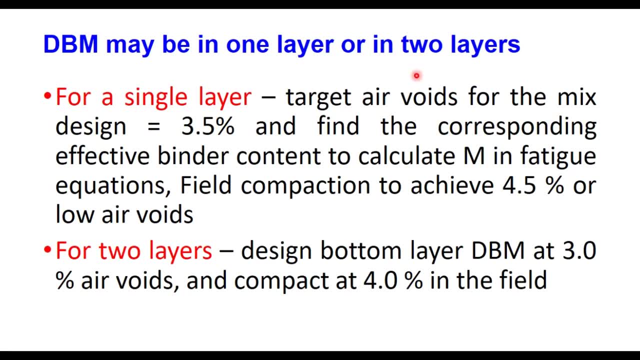 when you design the mix. And if it is not possible, then we can take from this table also. Now, if the resilient modulus value of the field mix is more than the maximum value indicated, either in one layer or in two layer, When you are putting BBM, that is the binder course. 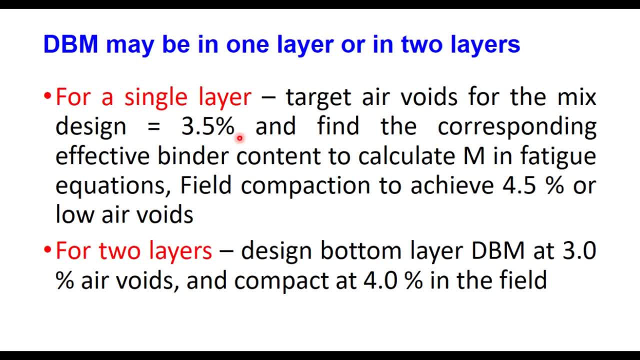 when we are putting BBM in a single layer. the target air voids for the mix design should be 3.5% and we should find out the effective binder content to calculate value of M in fatigue equation. Field compaction should be to achieve 4.5% or low air voids When. 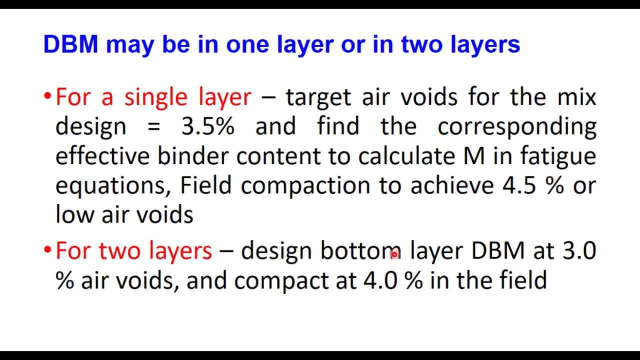 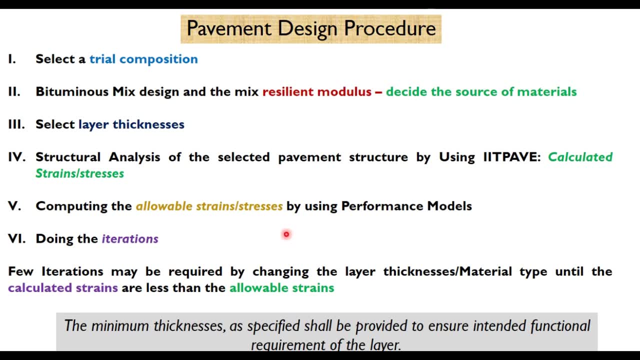 it is laid in two layers. the bottom layer, BBM, will have 3% air voids and that should be compacted at 4% air voids in the field. The procedure for pavement design as given in IRC code can be summarized in these six steps. 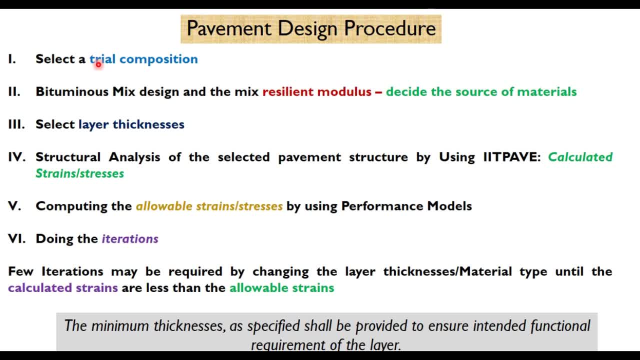 Select a trial composition and it should be based on the expected functional requirement of the layers. Then right proportioning of the mix, right proportioning of the mix ingredients and the design mix should be arrived at. As far as possible the resident modular should 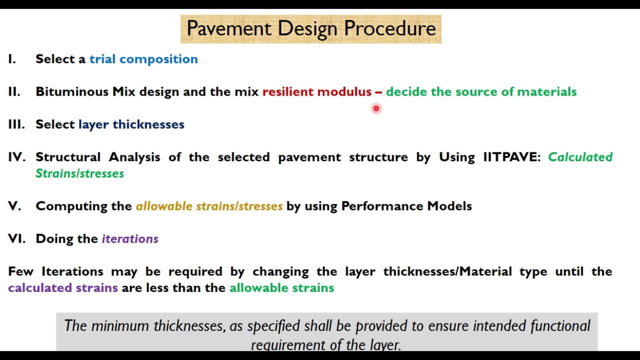 be determined in the laboratory, and if it is not possible, then we can take the value of MR from the table given in IRC code. Then we select the layer thicknesses. Trial thickness of various layers of the pavement will be guided by the experience of the designer, as well as minimum thickness required for. 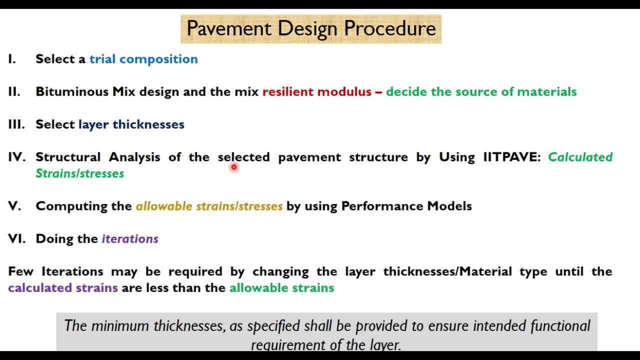 a layer Structure analysis of the selected pavement structure. by using IIT-PAVE and through this software, we calculate the stress and strain at desired points, at critical locations, and these stress and strain should be compared with allowable stress and strain by using performance models And if allowable strain is more than the actual strain stress coming. 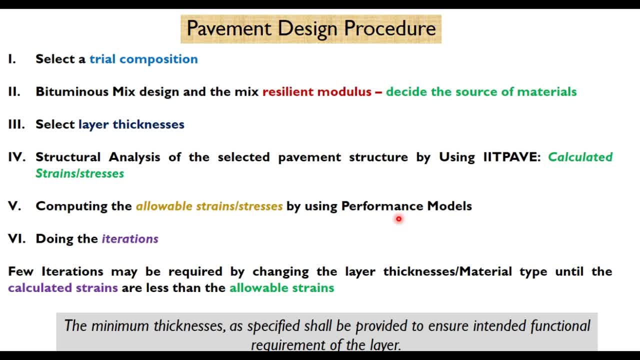 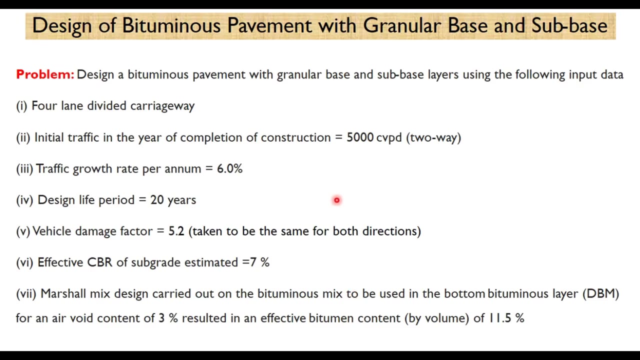 on the pavement, then the design is safe. otherwise we go for another iteration- And many times few iterations will be required- by changing the layer thickness or material type of the pavement until the calculated strains are less than the allowable strain. Let us take one example. An example is like this: that design a bitmes pavement with granular 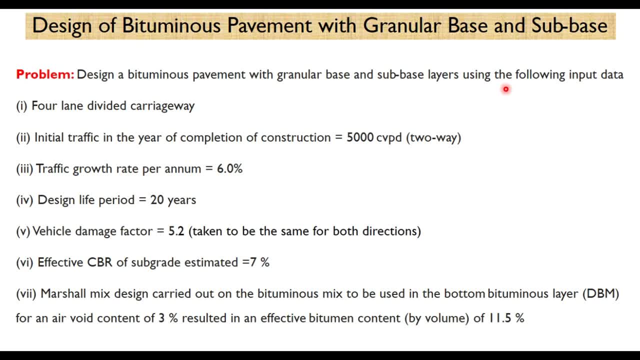 base and sub base layer using the following input data: See conventional type of pavement, say 4 lane divided carriageway, that will require 4 lane distribution factor, initial traffic in the year of completion of construction and the length distribution factor that will 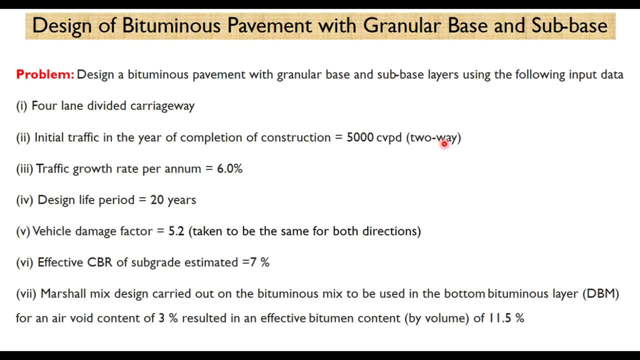 be 5,000 C, 2.3 kilometers. Each direction will be 5,000 C, b, p, d, потому both directions in a combination. The road rate value of the traffic: R 0.06.. 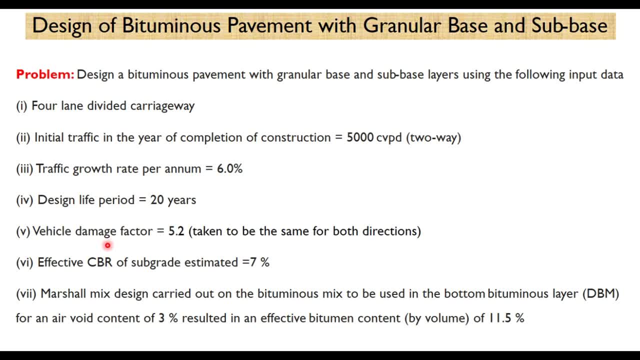 The design life is 20 years. the vehicle damage factor is 5.2.. The effective CBR of subgrade estimated at 7%. The marble mix design is carried out for the bottom bitmes layer, for the air wires of 3% And the resulting air effect between the construction and the construction. 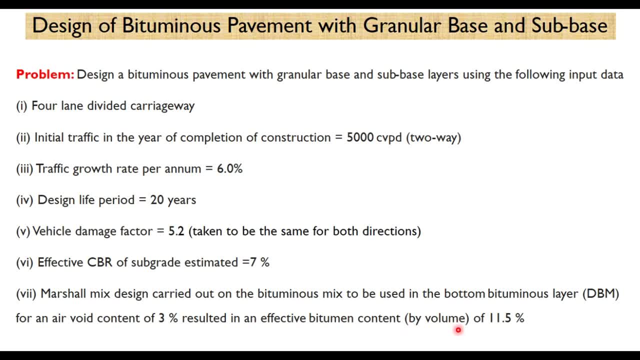 of the pavement. The people played often in the work. I took this example by comparing the facilities in the air and the ripple path. I took the result of 3 percent of the air between content by volume of 11.5%. Now these are required to calculate value of C and M. 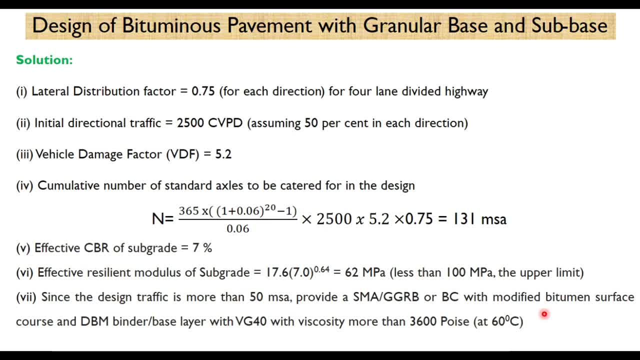 in fatigue equation. So the solution is like this: Lane distribution factor for a four lane divided highway is 0.75. Initial traffic in one direction will be 2500 CVPD. Vacant damage factor is given as 5.2 and therefore you can calculate the cumulative number of standard access to be. 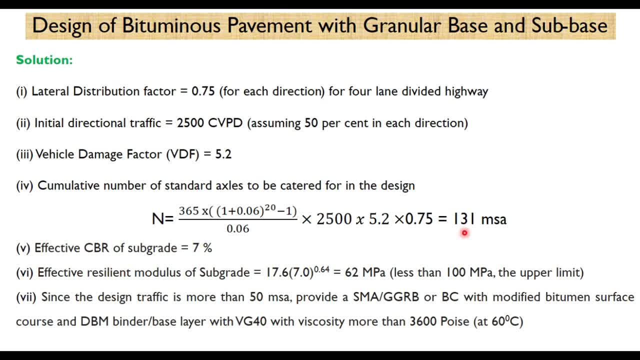 catered for the design and that is 131 MSA. CBR 7% effective resident modulus of subgrade for 7%: 17.6 into 7 to power 0.64, that is 62 MPa and it is less than 100 MPa. that is the upper. 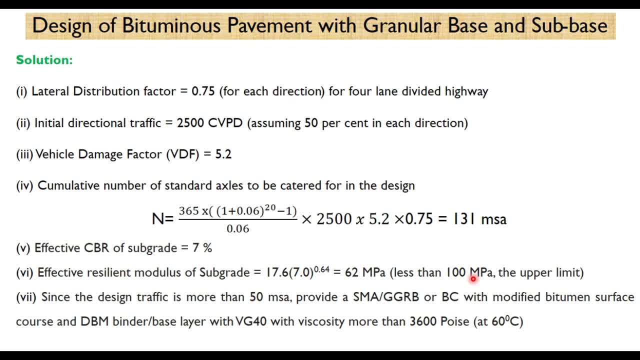 limit is specified in the code and therefore we will use 62 MPa as MR for subgrade. Now, since the design traffic is more than 50 MSA, therefore, we will provide stone matrix asphalt or this GGRB, which is gap graded, mixed with rubberized bitumen or bituminous concrete. that is the first row. 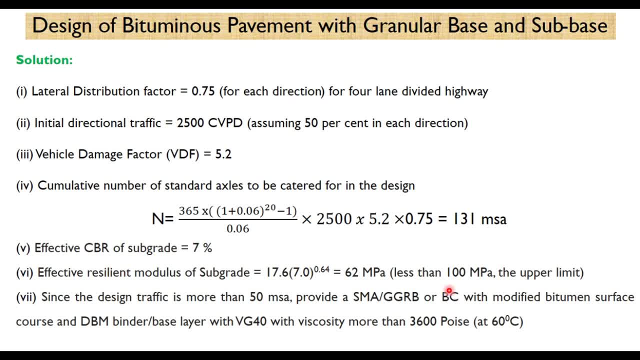 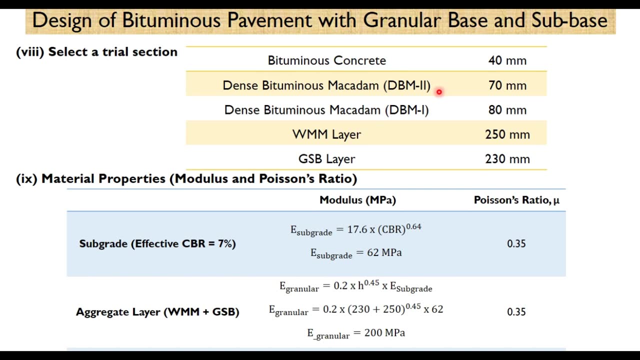 of the table with modified bituminous surface course and DBM layer with VG 40 with viscosity more than 3600 poise at 60 degree centigrade. Now let us assume this trial section, that bituminous concrete is 40 millimeter, DBM 70 millimeter and below that 80 millimeter binder. 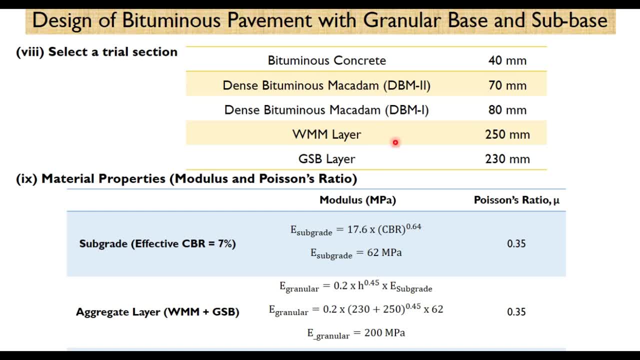 course, as a first layer, WMM 250 millimeter and GSB 230 millimeter, and for these thicknesses we can calculate the total thickness of the concrete. So for this thickness we can calculate the properties For subgrade. we have found out 62 MPa and Poisson ratio is 0.35.. For aggregate layer, 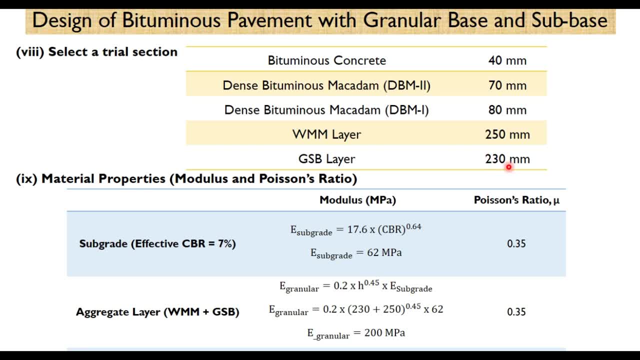 we will take combined thickness of 480 here. in this equation H is 480 and E support is 62. So you get E of granular material is 200 MPa and Poisson ratio is 0.35.. For HMA, for BC and 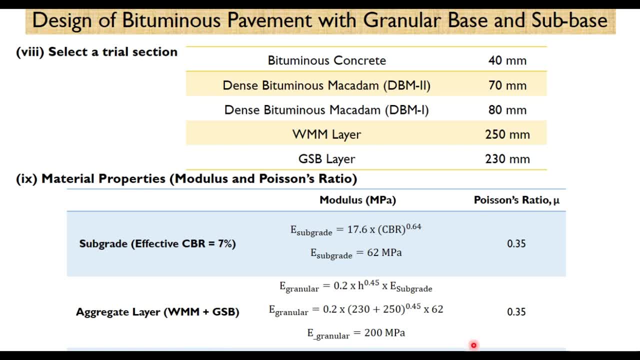 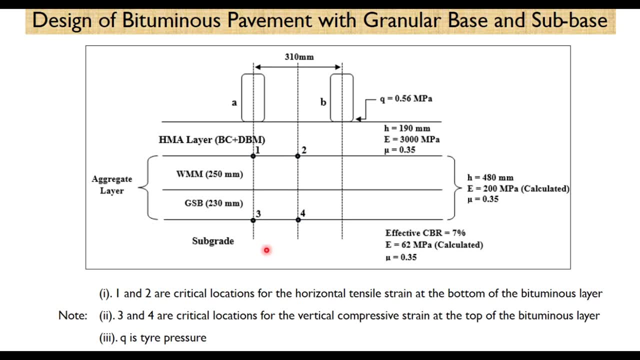 DBM, the value of 3000 MPa will be taken from the table. So this is the structure, this is the pavement structure. we have subgrade where effective CBR is 7%, E value 62,, MU value 0.35. then we have 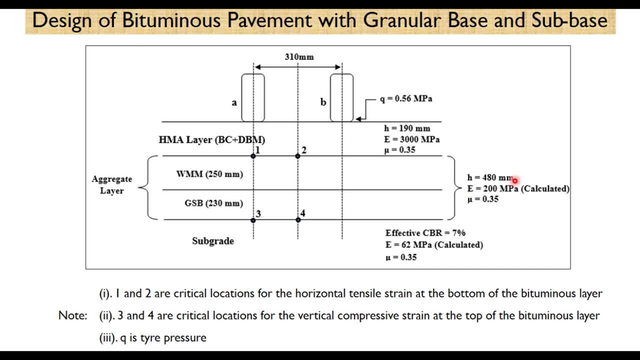 aggregate layer where combined thickness 480 millimeter, E value 200 and MU value 0.35, and above 190 millimeter E value 3000, MPa and mu value is 0.35.. So for this composition, these are four. 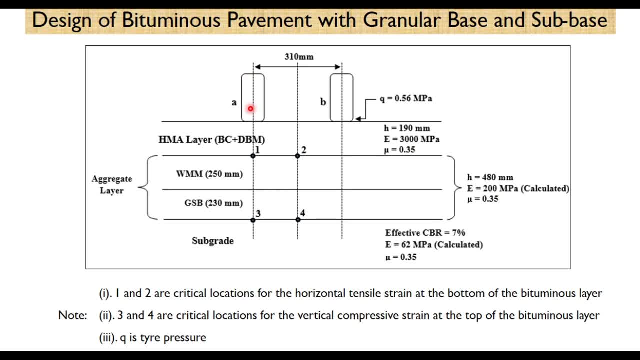 critical locations: One that is below the wheel, two is the center of the axle and three and four. One and two are below the bitmus layer and therefore here horizontal tensile strains are important. Three and four are at subgrade level and therefore compressive strain at. 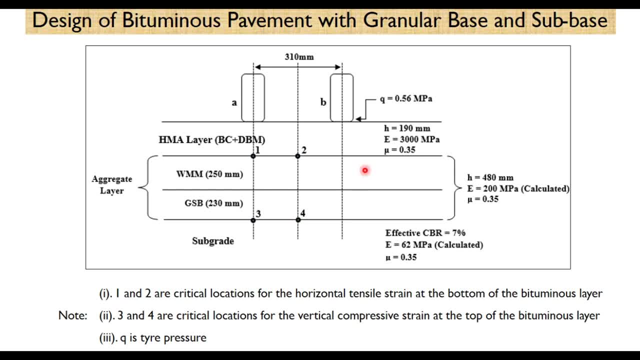 subgrade level are important, And Q is the tire pressure: 0.56 MPa. This distance between the center of the tire is 310 millimeter and therefore this 0.2 will be at 155 millimeter from the wheel load. 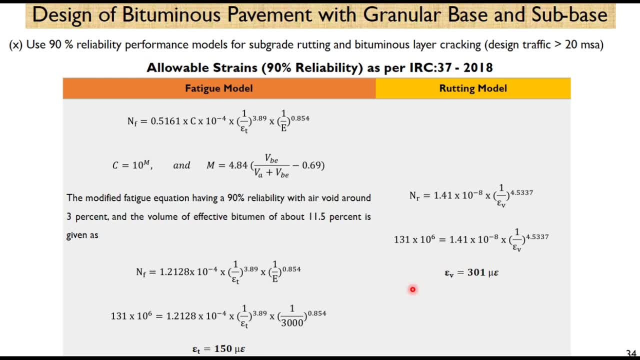 So with these parameters we can calculate the allowable strain at 90% durability as per IH 37.. For fatigue model, this is the equation. Here, C is a parameter which depends upon M and M depends upon effective boundary content and air wires. 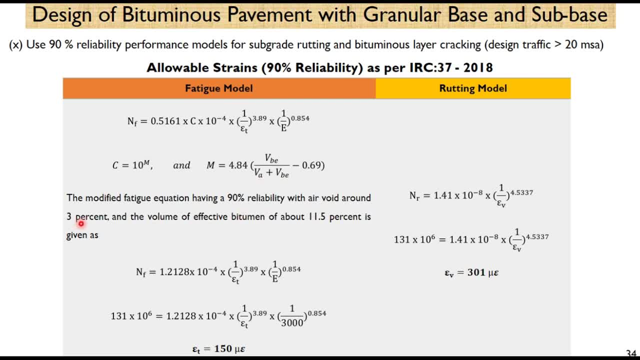 So if you put the value of air wires as 3% and VBE as 11.5%, you calculate value of M and from M to a value of C and put this value of C here. Now this equation is modified to this: 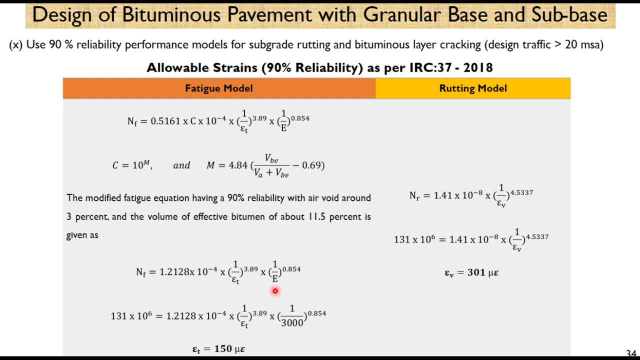 equation, And if you put value of E as 3000 and NF as 131- MSA- that is for design traffic- you can calculate what is the allowable strain. epsilon T, 150 micro amp. Similarly, for rutting equation, if you put value of M as 30, you can calculate what is the allowable strength. 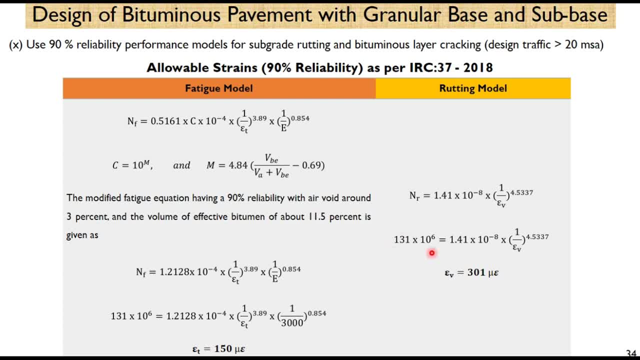 nR equal to design traffic at 131 million. you can calculate what is allowable compressive strain at the level of subgrade top, and that is 310 microns. Now these values allowable strain should be more than the actual strain coming on the pavement. 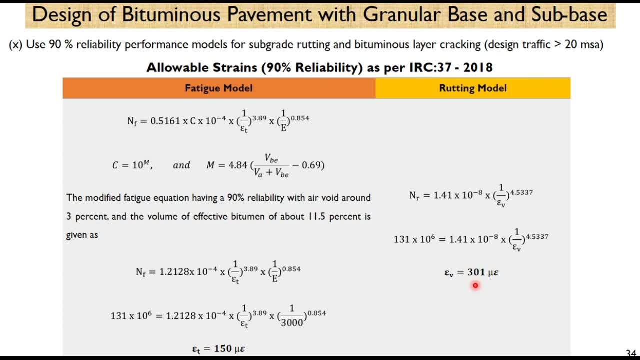 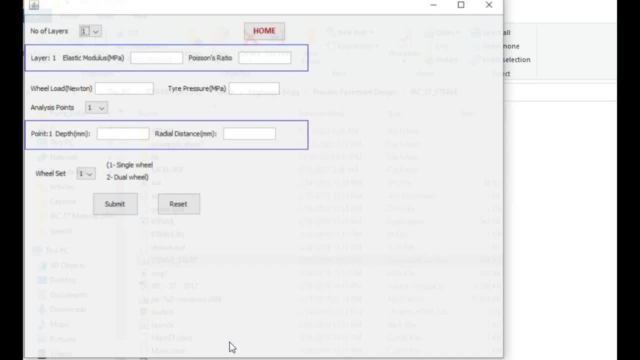 So we again go to IIT-PAVE to find out, for the trial section which we assumed, what are the strain values at critical locations. We again go to IIT-PAVE and design a new pavement section where you will see the number of layers. number of layers is 3 and 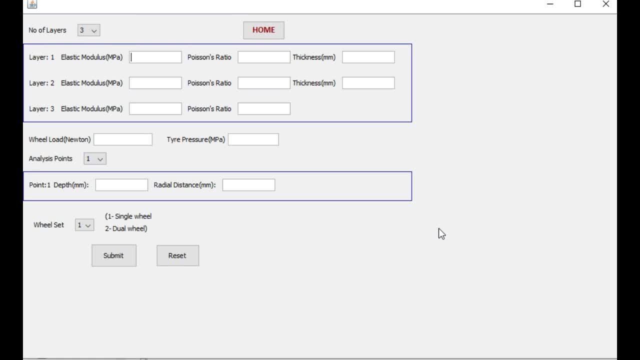 we need to put all the input data. for layer 1, the elastic modulus is 3000, Poisson ratio is 0.35 and thickness is 190 millimeter. For second layer, the elastic modulus is 200 MPa and Poisson ratio is 0.35 and layer thickness is 480. For third layer, which is subgrade, the elastic modulus is 62 and Poisson ratio is 0.35.. The V-load is 20,000 and Tire pressure is 0.56.. Now here we need the result at four points. The first point is below the bitmus layer, that is: 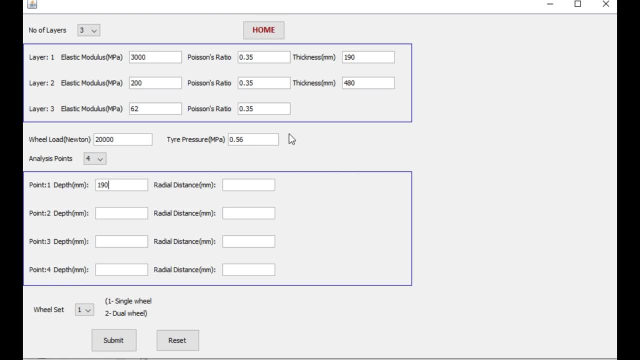 190 millimeter and below the V-load, the radial distance will be 0 and between the axle at the midpoint of axle the radial distance will be 155.. Point number 3 will be top of subgrade, That is, 670 millimeter total thickness of the pavement above subgrade and. 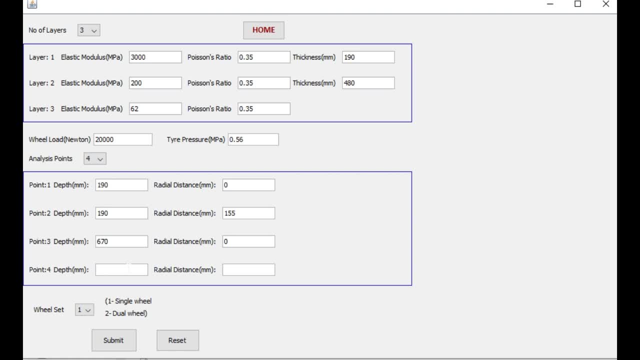 radial distance 0, that is, below the V, and 670 at a radial distance of 155 millimeter. The wheel assembly is dual V and we submit these data. Once you submit these data, then you can run the program and after that you can see the result. 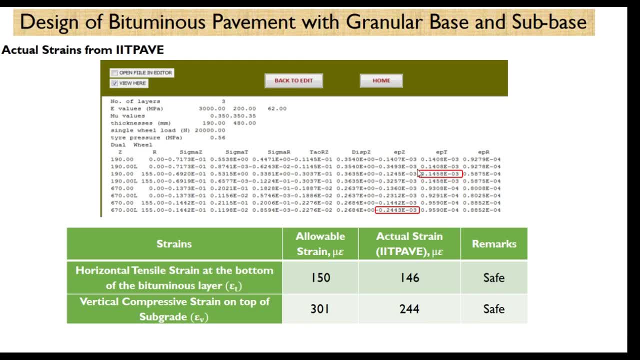 In this output. these values are critical. that is, epsilon t, tensile strain at bottom of bituminous layer and that is at the center of the axle, and similarly epsilon z, that is, compressive strain at top of subgrade soil and that is also coming at.